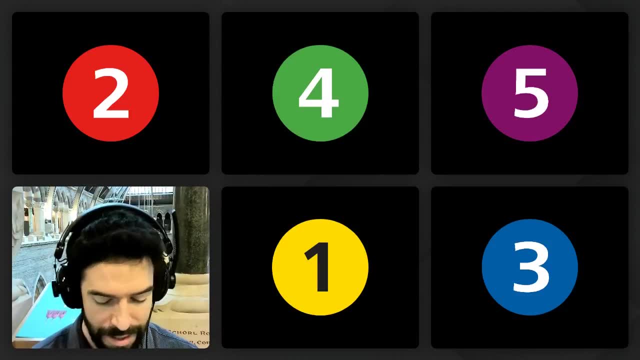 All right, welcome everyone to this session 3B from the 64th annual meeting of the Palaeontological Association. here live from the beautiful Oxford Museum of Natural History, and people are keep joining us right now. So this is session 3B and will be based on five talks of 12 minutes each. 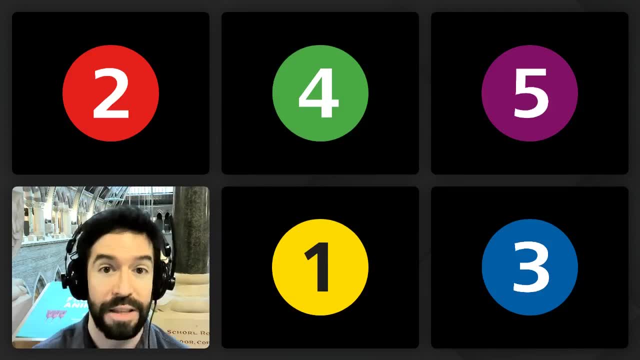 with three minutes for questions at the end of each talk and should you have any connection issues, please click the reconnection button at the top of your screens. and, of course, please use the chat to flag any questions that you have for the speakers. You do so by clicking on the. 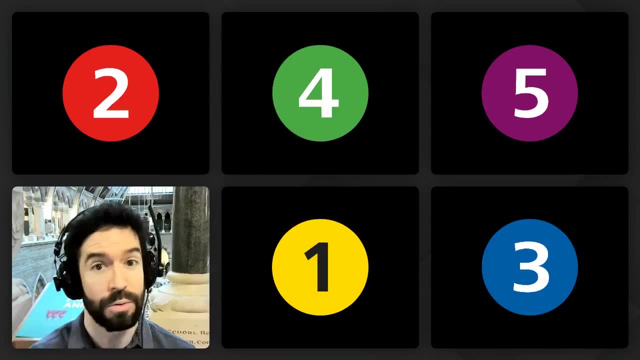 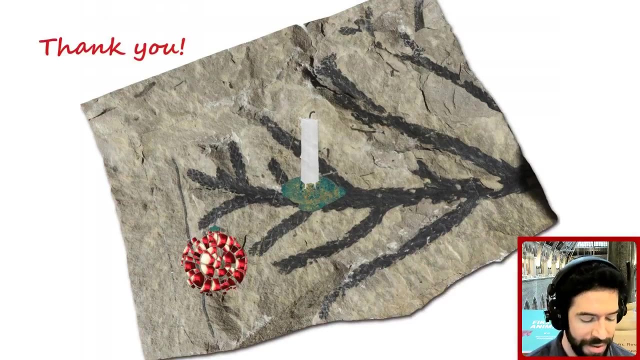 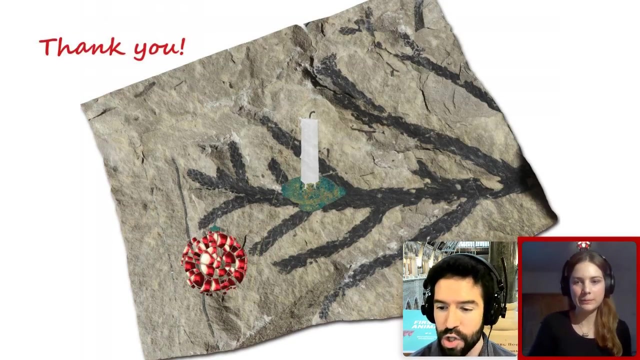 red circle at the at the right of your, of your, what you're typing basically, and we would select some of the questions for for the speakers, and the speakers can also answer to the questions after, after the talk, using the chat. Martha Gibson, Martha, are you there, Lovely? now let me switch the. 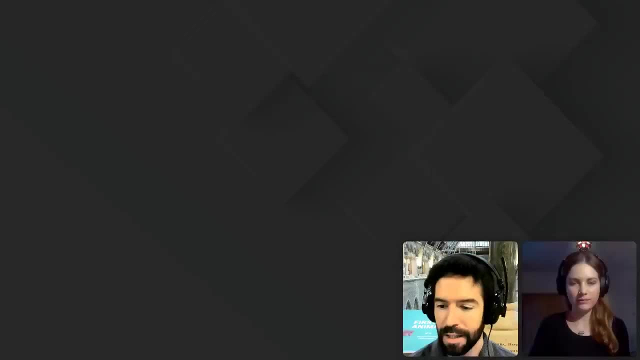 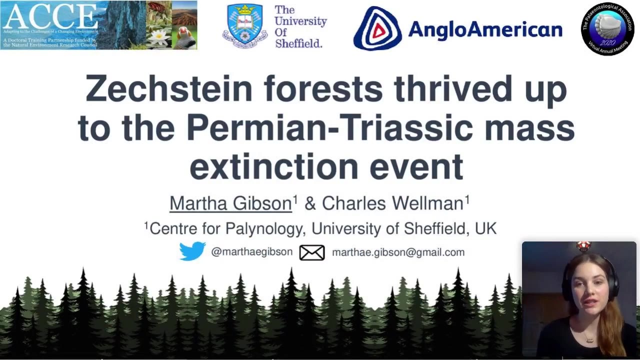 presentation charge yours and, all right, great, all yours. thanks. Thank you for that introduction. Today I'm going to be talking about some of the main results from my PhD project which I undertook at the University of Sheffield, where I was using palynology to reconstruct the Zechstein forests of central western Europe. 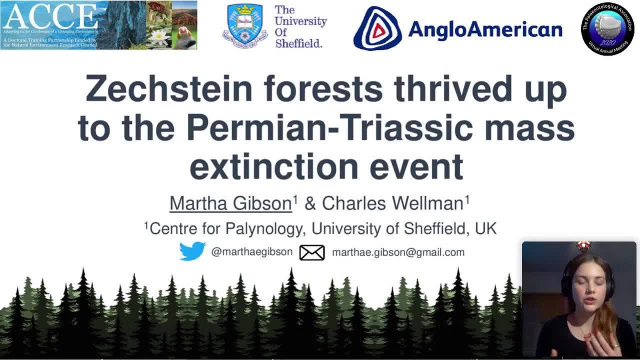 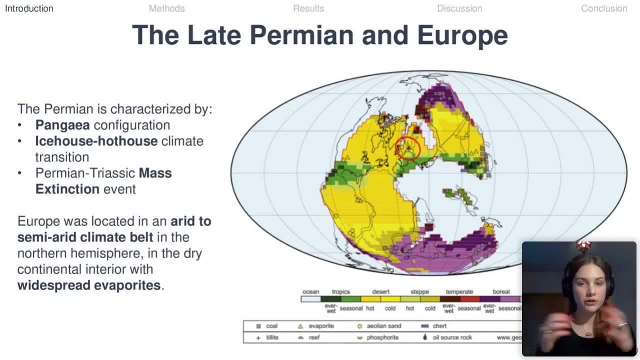 and in doing so I have made a new reconstruction for the region during the Lepindian, but I've also challenged some assumptions about deforestation as well at the end of Permian mass extinction. So we all know that the Permian is characterized by a Pangean configuration which created a lot of 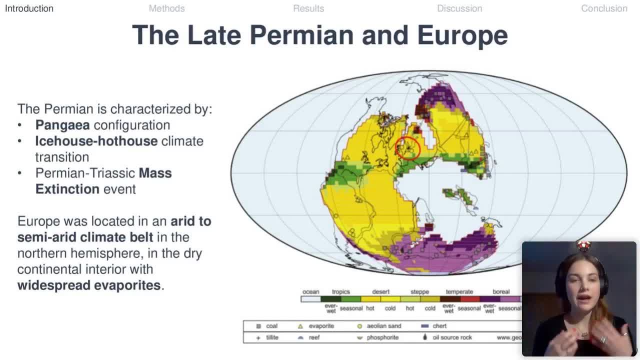 changes in the arid continental interior, the ice house, hot house climate chosen and, of course, the Permian trassic mass extinction event. but the responses of plants to this mass extinction that are still relatively understood compared to other groups. During this time Europe was located in the 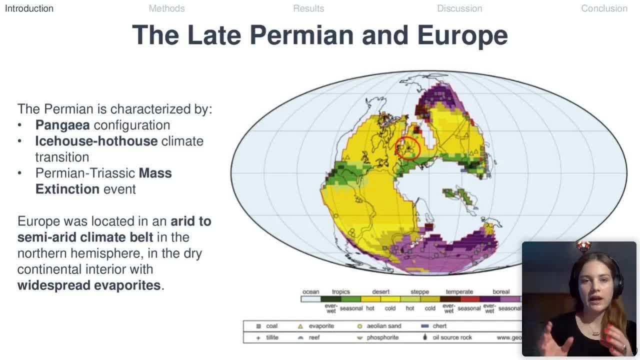 arid continental interior of the northern Pangea and in the paleo map you can see the red circle and that is our study location, the Zechstein sea- smack bang in the middle of Europe. The Zechstein sea is special because it deposited a massive amount of evaporites. 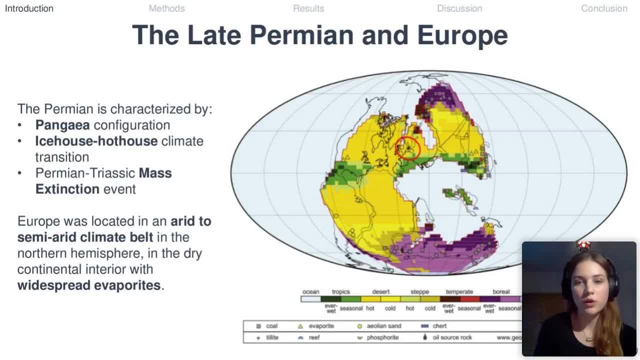 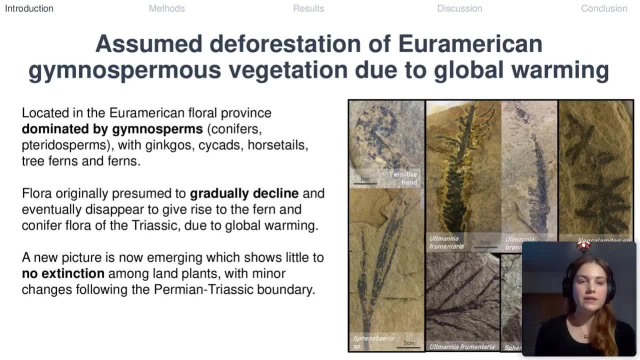 and is the basis for environmental and climate reconstructions of Europe for the Permian. So the Zechstein sea was located in the Euro-American floral province, which is characterized by gymnosperms and is dominated by conifers and the now extinct treedusperms. 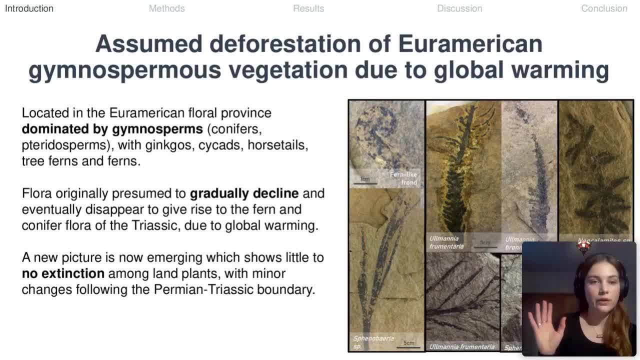 but you also see macrofossil evidence, like on the right, of ginkgos and cycads and horsetails, tree ferns and true ferns as well. But because of the global warming trends through the Permian and the impending mass extinction, it's been previously assumed that this vegetation gradually declined throughout the existence of. 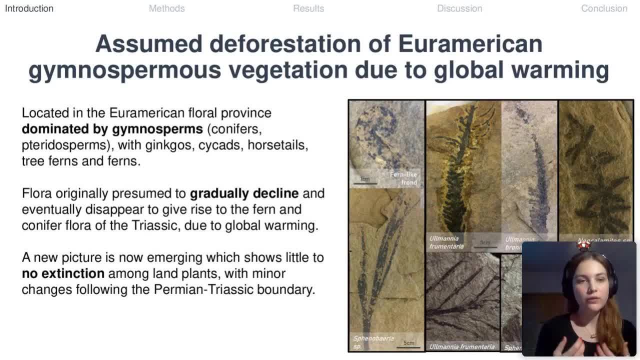 Zechstein to give rise to the fern and conifer flora of the Triassic, but in recent years we've had more of an interest in palynology and also paleobotany across the Permian-Triassic boundary, and this has really changed our understanding and is showing that there wasn't 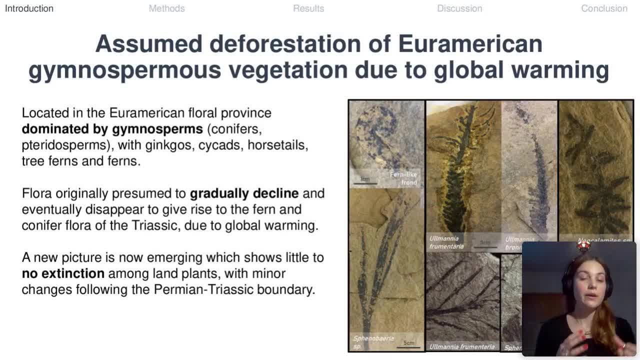 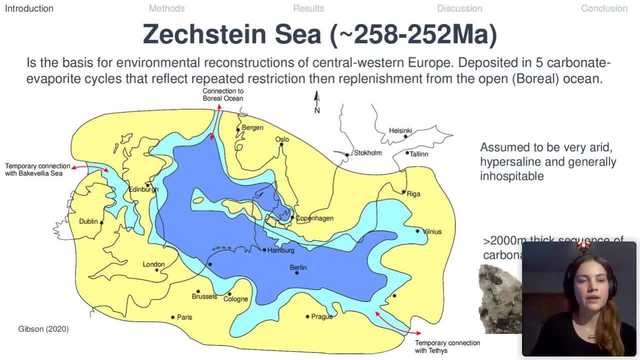 really this mass extinction among plants, like we believed, and there are minor changes following the Permian-Triassic boundary, not necessarily in the run-up before. So here we have our Zechstein sea. It is deposited in five carbonate evaporite cycles that reflect 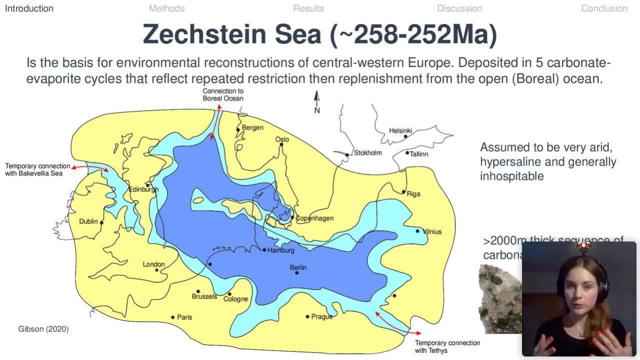 repeated restriction and then replenishment from the open ocean, which was the Boreal ocean at the time, to the north. Its deposits can be found along the east coast of England, which is where I have been studying the Zechstein, but it's found underneath the North Sea and also crops out. 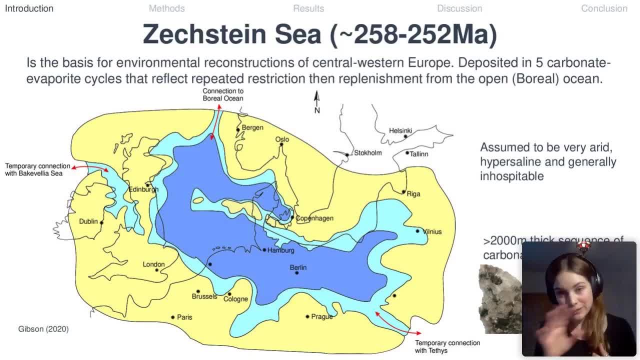 in Germany and Poland as well, and my face appears to be covering my lovely pictures of my evaporites. but it deposited over 2 000 meters of these evaporites and carbonates and because of their sheer volume the environment is assumed to be generally arid, hypersaline and 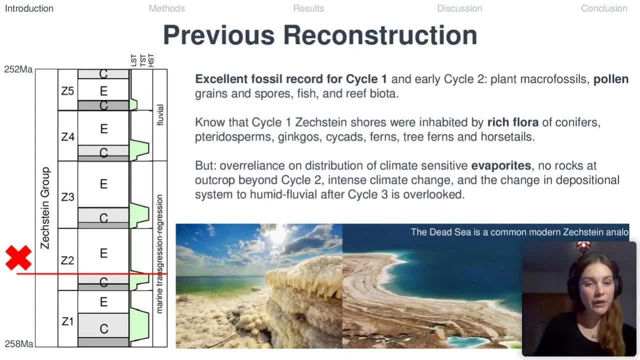 quite inhospitable to plant life. But there are some issues with this reconstruction. First and foremost is that at outcrop in the UK the rocks are missing from cycles three, four and five, so we only have a fossil record for cycles one and two, and this has meant that 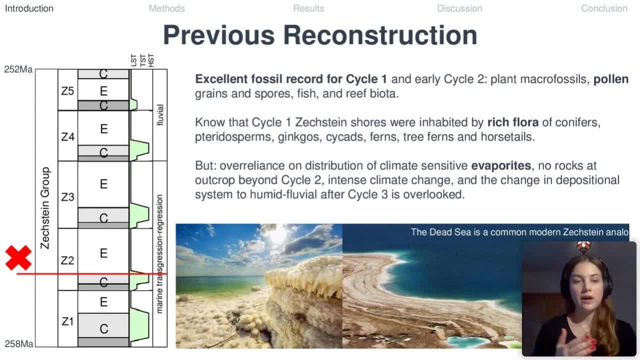 we assume that the vegetation and fauna disappear or go extinct after cycle two and the rest of the Zechstein is reconstructed a little bit like the Dead Sea. The second oversight is that there's actually a change in depositional system between the lower Zechstein. 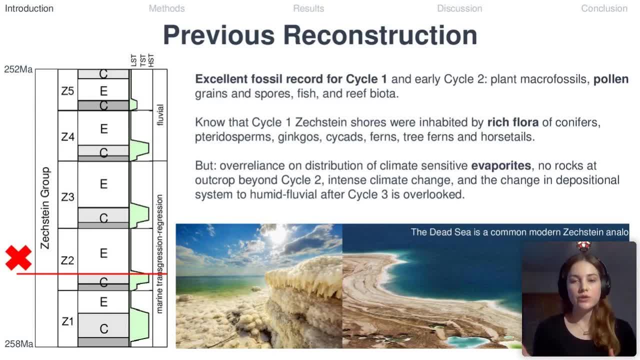 cycles one, two and three and then cycles four and five. At the beginning of the Zechstein we have a marine transgression regression depositional system, but there's evidence of a global regression between cycles three and four, meaning that our fourth and fifth cycles are actually this humid. 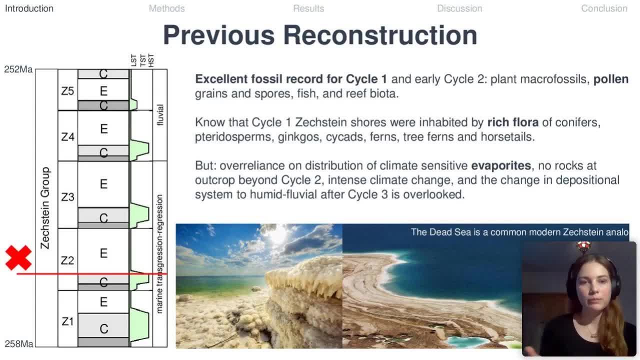 fluvial depositional system, which is quite favourable for plant life In general. previous reconstructions are based on an over-reliance on the distribution of the climate. so we know that there are no rocks. so there's a missing fossil record. We know that there was. 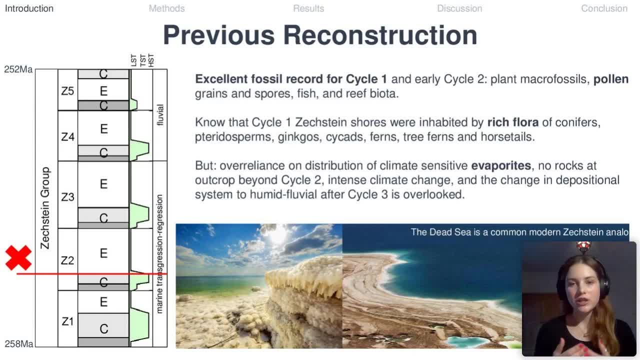 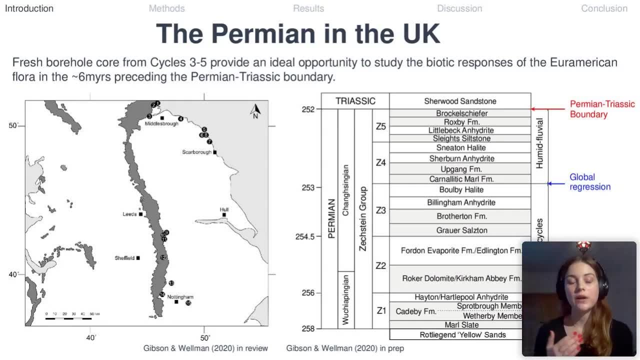 intense climate change happening during the Permian and the change in depositional system has been overlooked. So for my PhD I got access to freshly drilled borehole material from Anglo-American which passes from the top of the Zechstein at cycle five down to the vaporites of the second. 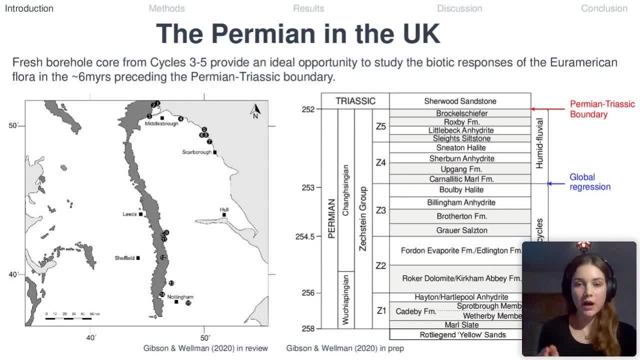 cycle And these boreholes come from the country around Scarborough in West Yorkshire, but the Zechstein in the UK actually pops out from Northumberland all the way down to Nottinghamshire, representing the sea's most western extent. So the environments that I am effectively sampling in are marginal Playa Lake type settings and in the stratigraphy on the right. 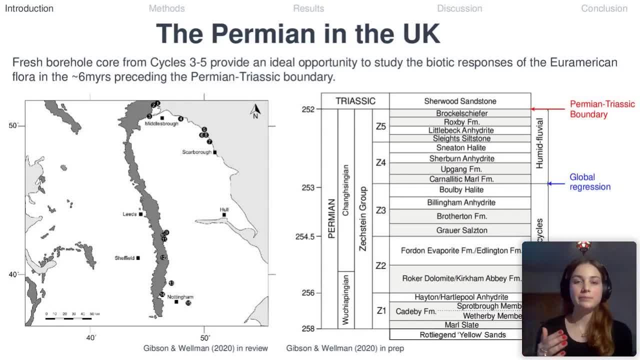 I've shaded the carbonate phases or formations and you can see how each cycle is divided into a carbonate phase, which represents the carbonate phase, and the stratigraphy on the right. This represents our marine transgressions and our system, high stands and the evaporites which 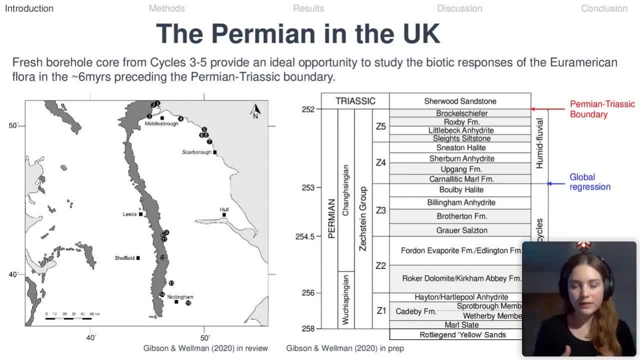 aren't shaded. they represent our evaporative phases. so system low slams and marine regressions, and these cycles get smaller and smaller as you go up the sequence and this reflects the ever shrinking volume of the sea. and really when we get to cycles four and five, 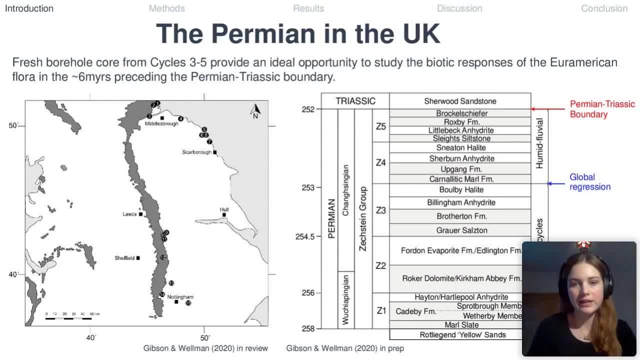 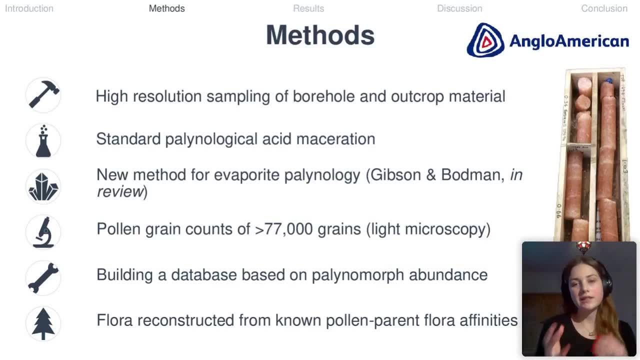 this the sequence is very, very condensed because we don't have marine influence anymore. So I undertook high resolution sampling of both borehole material and I supplemented my borehole material with outcrop material to capture the first cycle. My samples are processed using standard panzeological acid maceration techniques, but I also developed a new method for extracting. 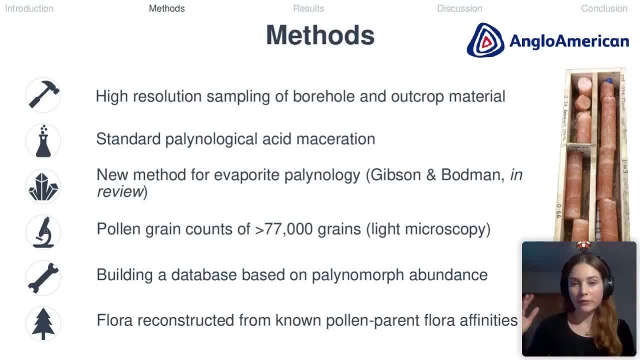 the plinomorphs from evaporites, and this was to really flesh out my sampling range but to also see if I could study the biotic responses of the vegetation in these really intense periods of evaporation. I then did a quantitative approach where I counted all my pollen grains. 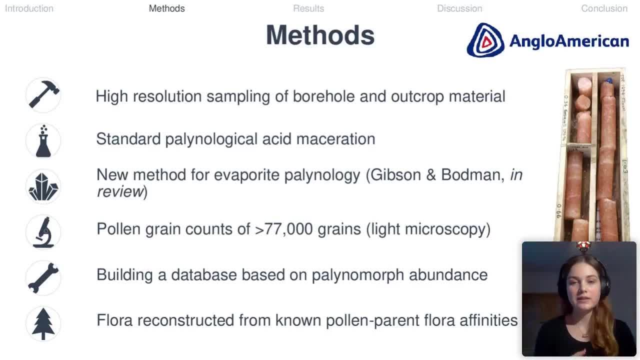 and then I composed a database based on plinomorph abundance and I reconstructed the flora using known pollen, grain, parent plant, floral affinities. So we have this sequence-wide picture of the zechtein, which has never been done before, at least for the UK, meaning we can look at biotic responses. 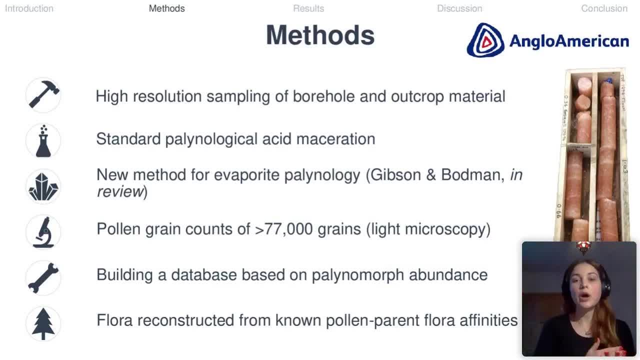 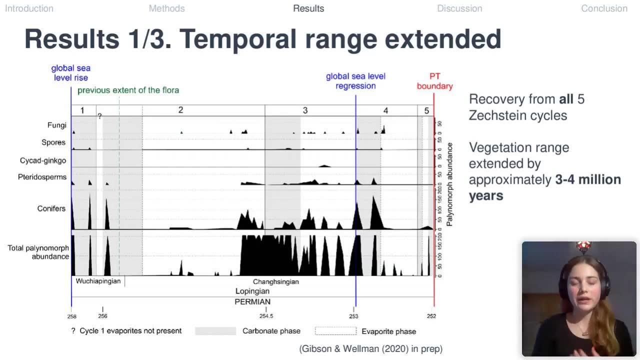 both across the overall zechtein, which reflects our permanent climate change trends, but also within individual cycles, to see if we can tease out any responses to this cyclic increases in aridity, but also salinity. So I'll be breaking down the major results of my research into three parts based around this graph. So this graph shows the 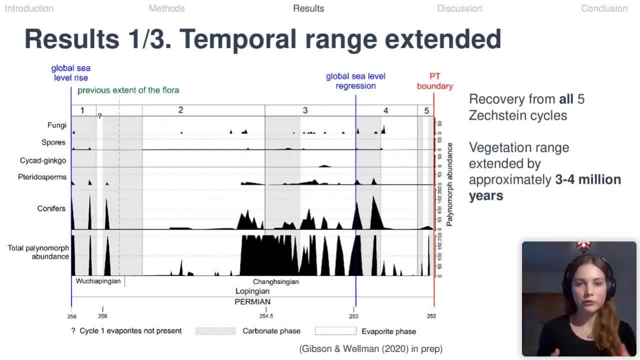 abundance of plinomorphs, divided by parent plant group throughout the five cycles of the zechtein. The green dotted line here is very important because that represents the previous extent of the flora from previous reconstructions. it supposedly disappeared at the beginning of cycle two but as you can see from the data here we have recovery from all five zechtein cycles. 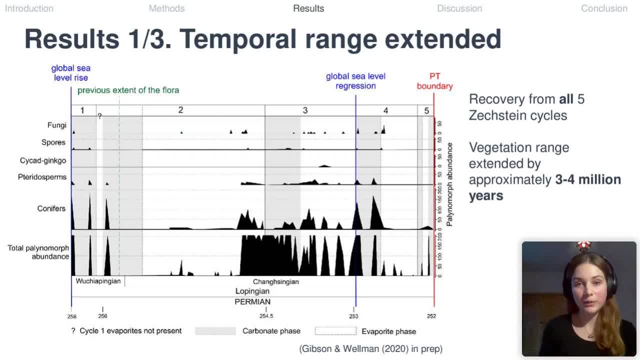 and this significantly extends the range of the vegetation at the end of the Permian by an extra three to four million years. It is present right up to the Permian-Turassic boundary. Secondly is about the nature of the plinomorphs and their relationship to the zechtein. So I'll be. 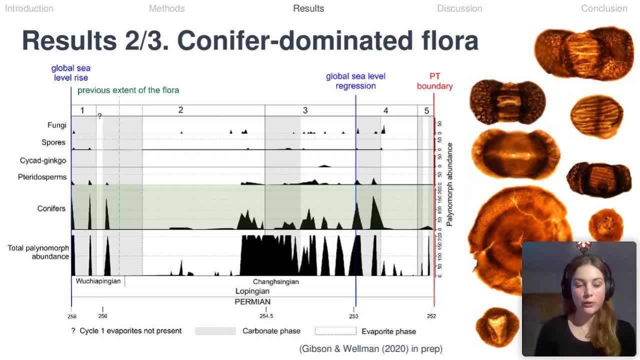 going over the nature of the vegetation. We know from the macroflossal record that we have mostly conifers and toreda sperms, and this is exactly what is reflected in the microflora. So conifers are consistently the most abundant vegetation throughout the zechtein. They are always the most 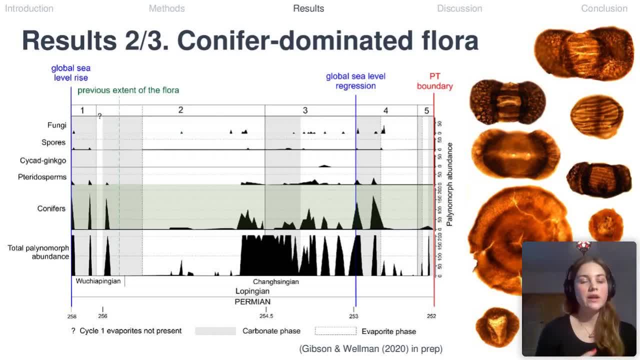 abundant. Tereda sperms are the second most abundant. but our sycas and ginkgos, our tree ferns and true ferns occur at very, very low abundance. They appear to be a minor component of the zechtein. The marine influence from foraminiferol test linings and acrotox was very 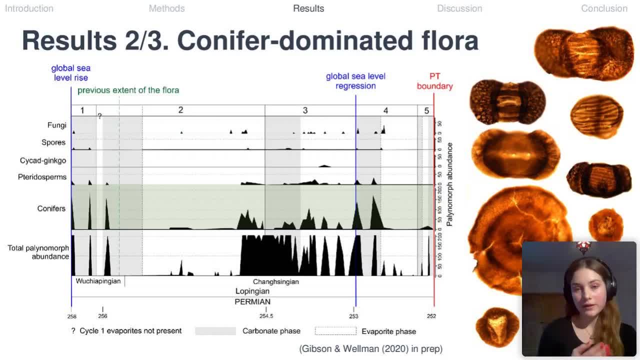 very minimal and, interestingly, our fungi- and this is Reduvia spironitis- occurred at very low abundances throughout the material and we don't see this mass occurrence. that is often described from other pt boundary studies as well as other mass extinction panelology studies. 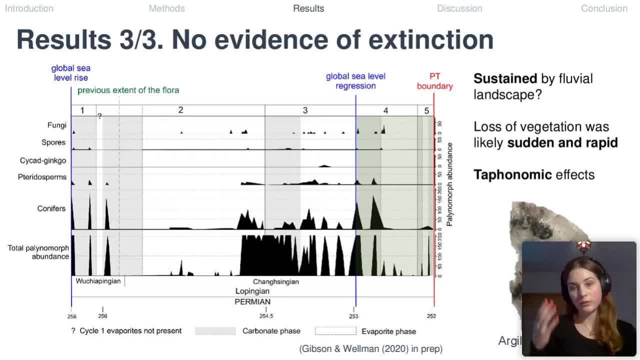 So one of the major results is that we appear to have no evidence of the so-called plant mass extinction and we do have this blip throughout the evaporates in, especially the second cycle, and there's intermittent recovery in this third cycle, and this is due to salting, and this is where 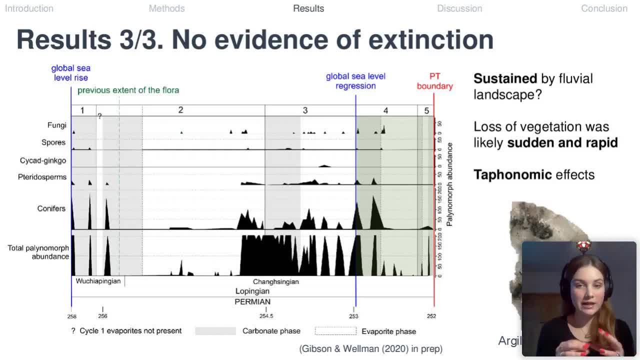 evaporates, precipitate at such a rapid rate that they dilute the concentration of any material that's trapped inside. So we know this from microbiological studies, we know this from astrobiological studies, but also it very much happens in palynology as well. and what is perhaps 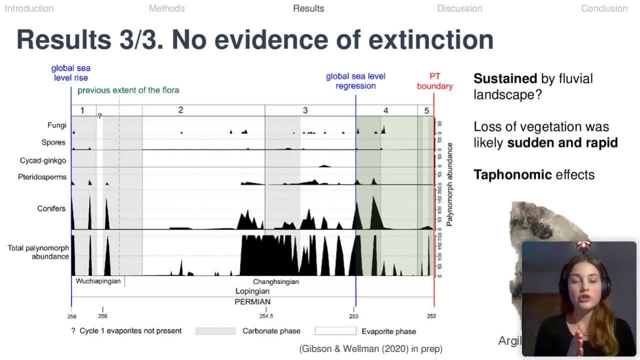 happening is that at the change in depositional system in cycles four and five, we have this fluvial landscape and perhaps this is what is sustaining the vegetation despite the climate trends in the upper Permian, and there does appear to be a slight decrease in vegetation. 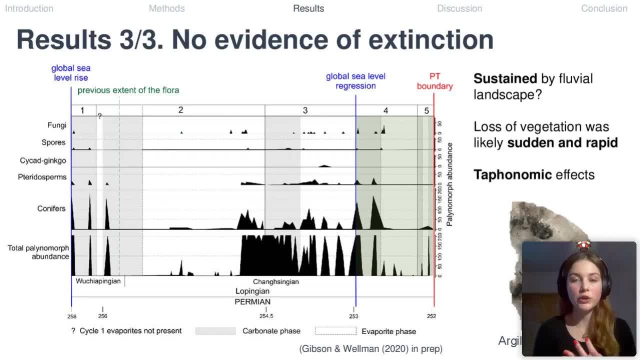 and this could reflect the true nature of the vegetation. it could indicate some sudden or rapid loss of vegetation. but it could also be a taphonomic effect, because the cycle five lithologies are dominated by oxidized red beds, which are notoriously bad for recovering palynomorphs. 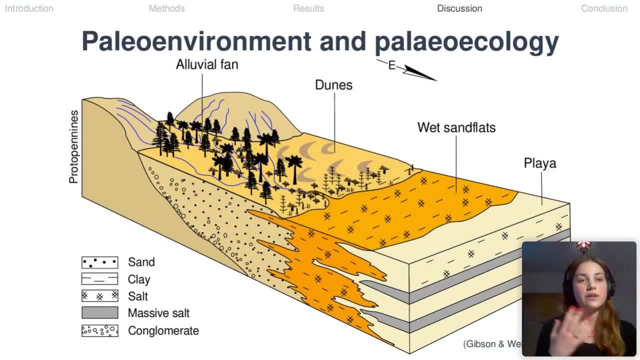 So, based on the lithological evidence and the palynology, this is a very basic reconstruction of what we think the uppermost search line would have looked like. We have no marine influence at this time, so we have a player lake type setting. we have some saline sand flats. 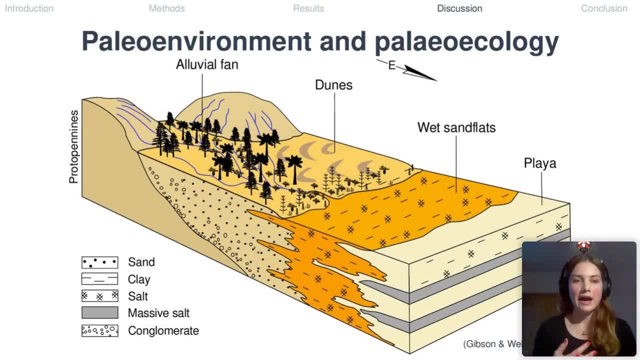 and then we have an inland alluvial flan type flora, and although our assemblages are dominated by conifer pollen grains, it's possible we do have a transport or a taphonomic bias from the inland fluvial system out into our depositional area. and 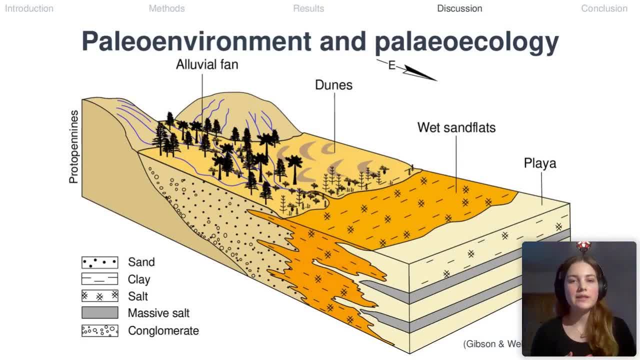 there is one disconnect between the macro and the microfossil record, and this is that we don't see any horsetail pollen in our assemblages, and I think this is probably because they're just too fragile and they're just not preserved. so it just goes to show. 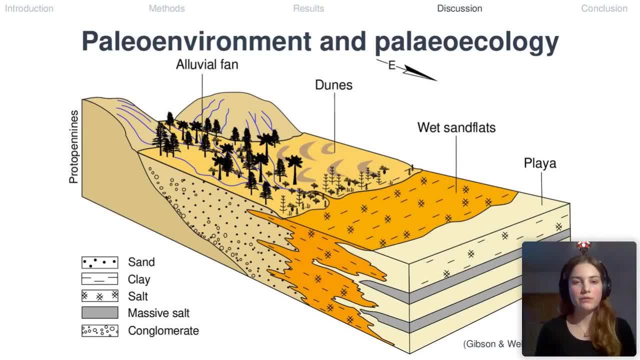 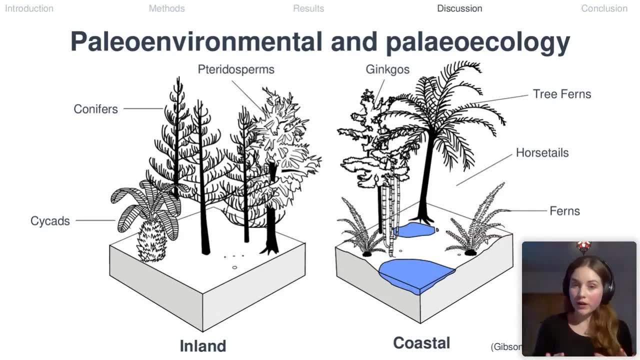 that there's still some things we can't really quite tie down about the Zetschstein flora and that we shouldn't be reading the palynology record quite so literally. But we can group our vegetation into two very broad categories that also have some intermediary as well. so in our arid 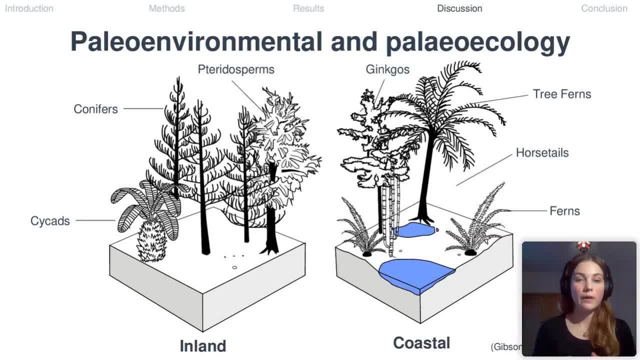 areas and our inland areas, we have plants that are slightly more xerophytic, adapted, so like our conifers, in slightly wetter patches in the inland area we likely had our Torridus ferns with the slightly thicker cuticles, and intermediary flora based on cycads and ginkgos, and tree ferns. 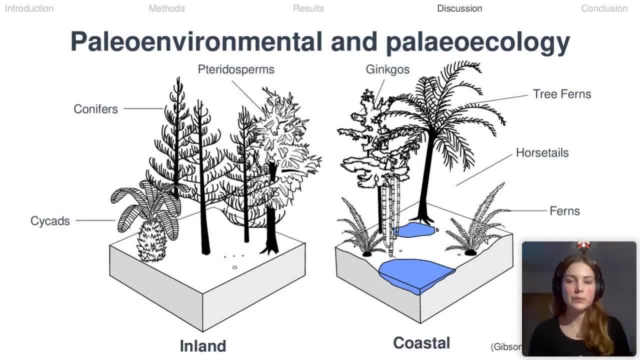 could have lived in more wet coastal areas, but also wetter patches inland as well, and we would have had a coastal flora of your wet loving plants, like your horsetails and your ferns. We are very good at living in harsh, stressful climates, including saline ones. 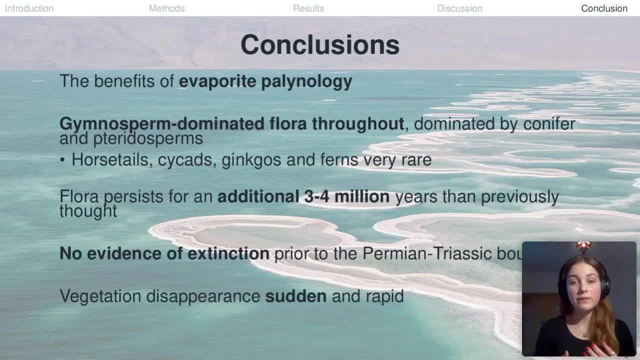 So, to conclude, this study really showcases the benefits of evaporite palynology and their exceptional preservation potential. We now know that the Zetschstein flora persisted for an additional three to four million years than previously thought, and it was gymnosperm dominated, like the macroflora record suggests, but it was also conifer and Torridus sperm dominated. 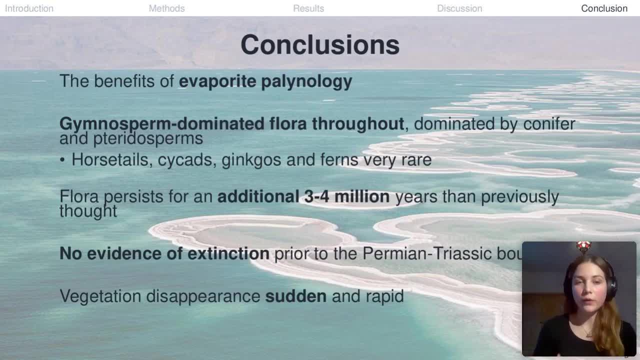 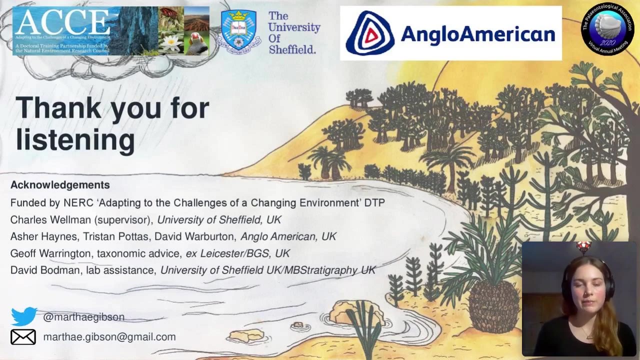 throughout. We don't have evidence of a deforestation in the landscape really prior to the Permian-Turassic boundary and if there was deforestation before the Turassic it was likely very sudden and rapid. So thank you very much for listening and I'd like to acknowledge the NERC ACPDP for. 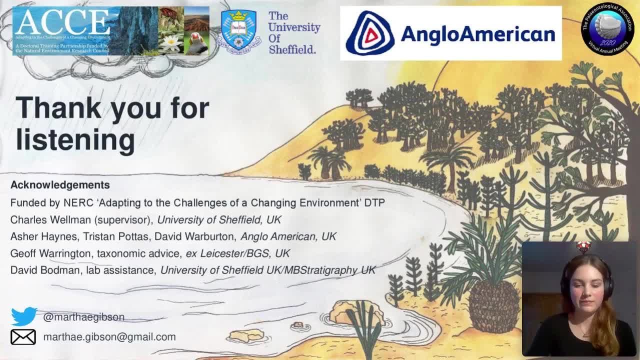 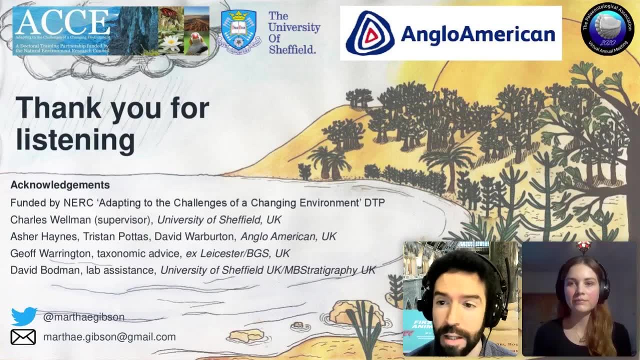 funding this research, Thank you. Thanks so much, Martha, for your talk and please, we have a couple of minutes for questions, so please keep them coming up in the chat. We have a couple of times now before we close one. you might have, uh, answered a bit. some of you talk about some of the biases, but margaret was 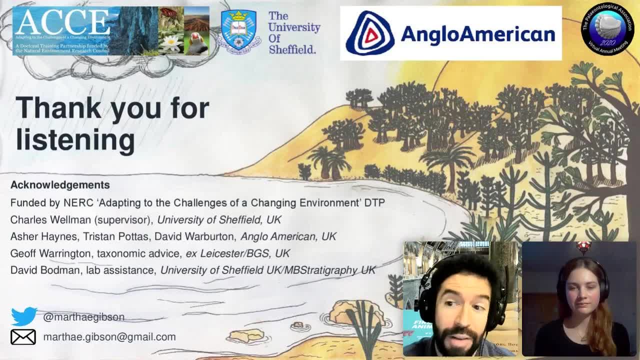 wondering: do you think that ferns have low or have a low abundance in general, because they were under understory plants biased against in your depositional settings? yes, i think that's very likely because our assemblages are dominated by wind dispersed pollen grains, so they're getting. 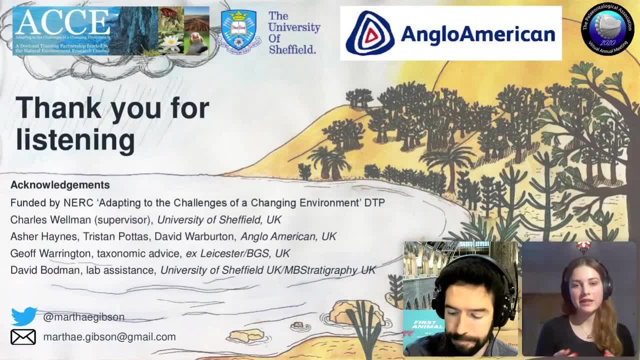 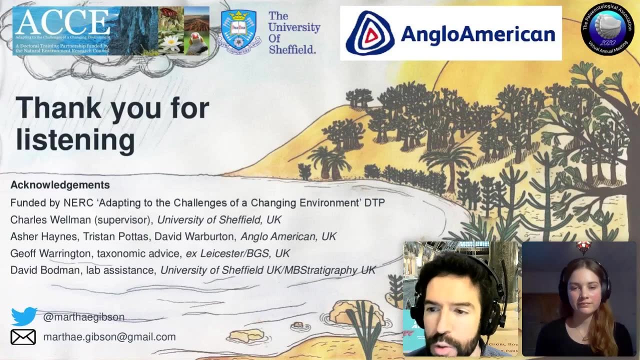 blown out across all the other vegetation and landing in the sea, and if it is a more arid environment, perhaps we're not getting so much um of our understory washed into the sea at the time. uh, another uh question here: do you find anything um building a logical across the pt boundary, any information and that you can extract from? 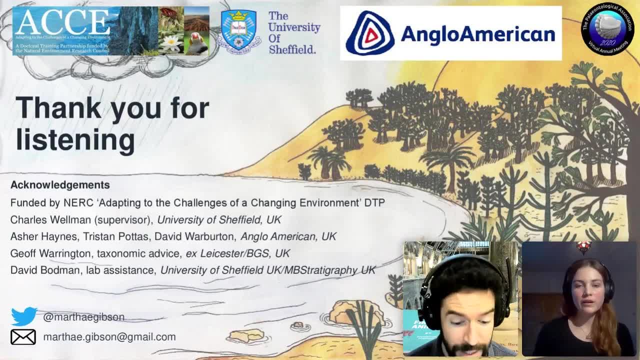 palynology in that boundary, the pt from the chromotriassic, from the zetschstein. no, in the uk it cuts off right at the pt boundary, but in germany and other parts of the zetschstein basin the zetschstein actually ends into the earliest traffic. but again. 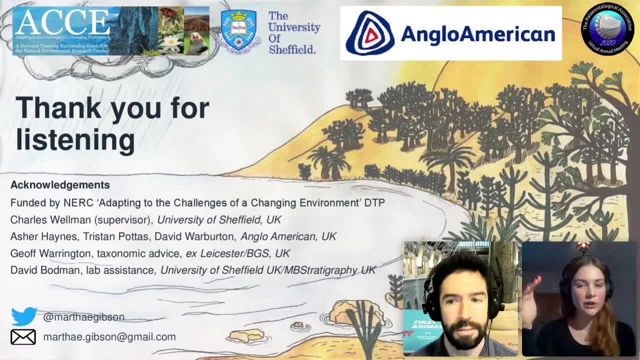 we have this issue of massive amounts of red beds, so we don't actually recover very much at all. so i can't say anything definitive about patterns across the pt boundary in the zetschstein great. all right, well, uh, um, feel free to answer some of the questions that. 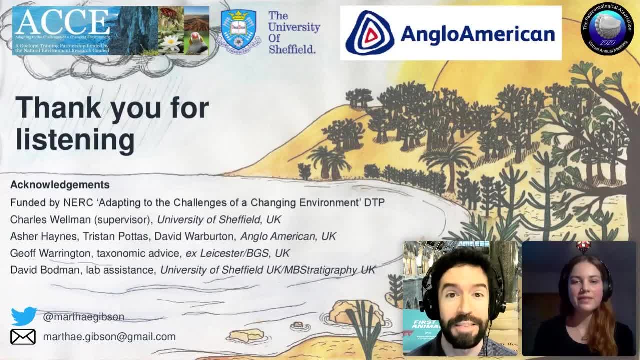 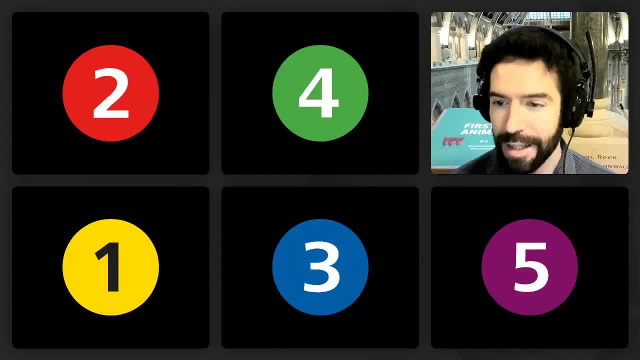 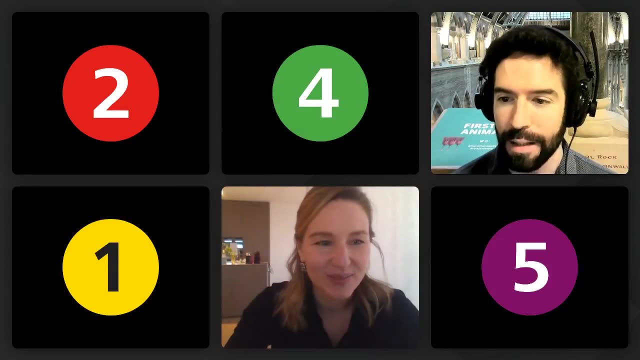 the extra questions that are going to be popping up in the chat for you, martha, thanks. so much thanks, and now the next speaker is lara shishio. lara, please, if you are there, connect your uh. all right, we have lara with us and i will upload your talk right now, and it's, the stage is yours, thank you. 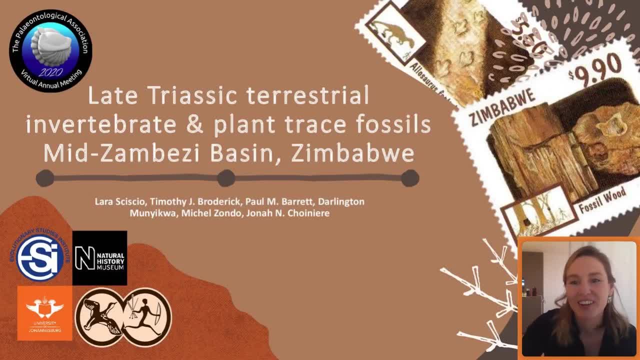 hi everyone, thanks for tuning in. i'm going to be discussing some field work around lake kariba in zimbabwe's upper trassic, lower jurassic upper crew group and specifically highlighting some of the invertebrate and plant um trace fossils that we have found in the mid-zambesi basin. oh i, i'm sorry, i can't. 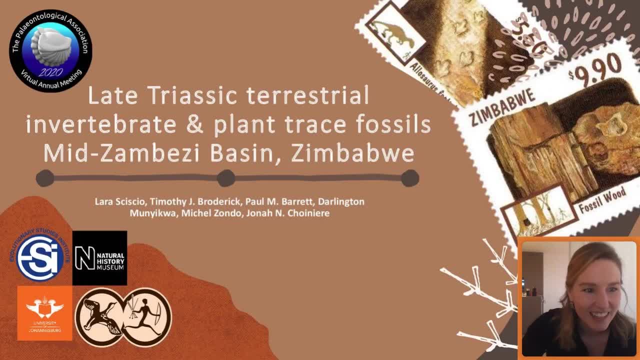 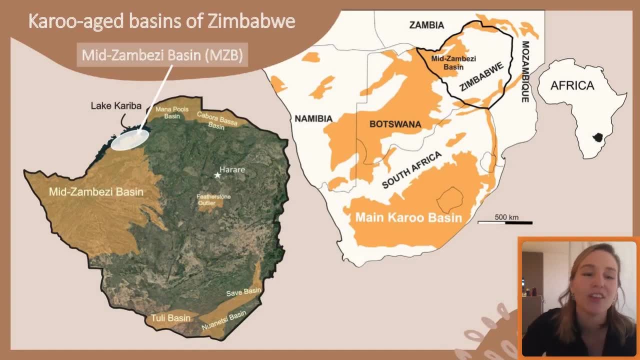 change the slide. ah, it's delayed. sorry everyone. i changed it for you, so let me know if you keep having issues. that would be wonderful, okay, so our work is based, as i said, in the mid-zambesi basin, which is one of several crew age basins in zimbabwe. crew-aged basins are roughly heinve with the formation and deposition. 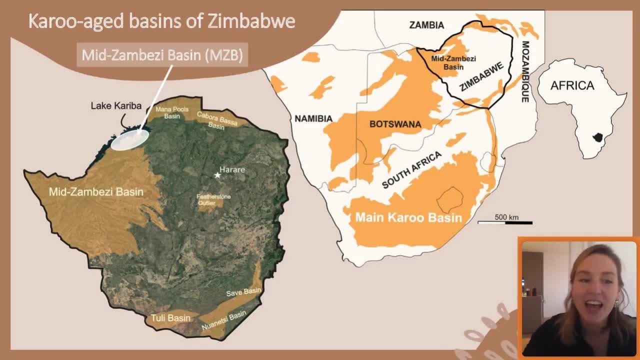 of the more well known main crew basin of south africa in lissias two, and the main crew basin- i mean the mid-zenbisi basin, as you can see in the um figure on the far left, is the largest and most extensive of the crew-aged basins in zimbabwe and in particular, our field work has been based in. 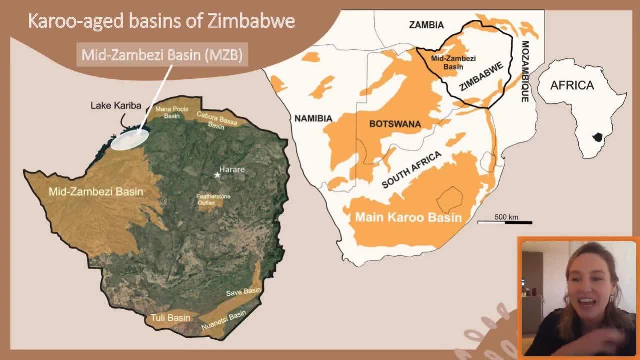 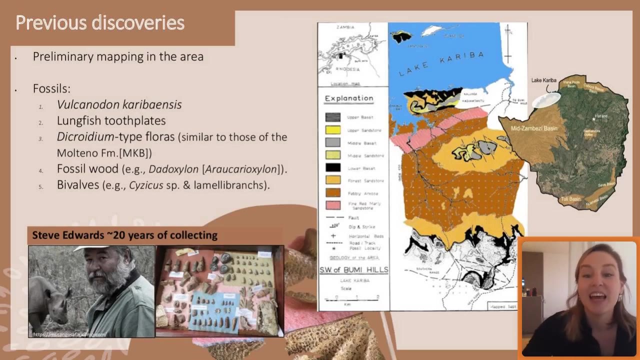 on where that white circle is in the northern end of the Zambesi basin and along the southern margin of lake ощiieba. Next slide, please. Previous work in the Upper Karoo Group. so the late Triassic and early Jurassic of the Mid-Zambesi Basin has largely been achieved in the 1970s. So there was some. 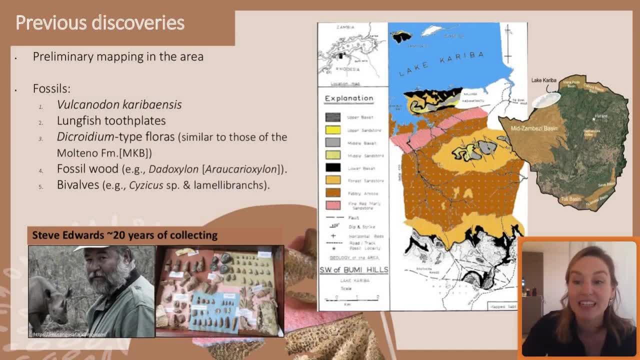 prelim field mapping and several fossil discoveries, most famously of the primitive sauropod Vulcanodon caribouensis. In recent years, and at least for the last 20 years, Steve Edwards from Asanga Safari Camp- and you can see him in the bottom left-hand corner of 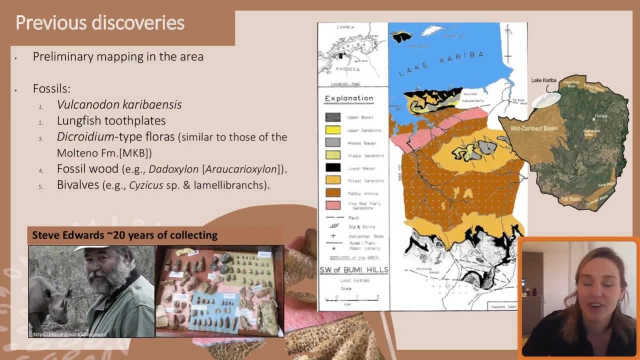 your picture has been an avid collector and curator of fossils found in and around Lake Kariba, and he first alerted colleagues to the potential, wealth and the necessity for new exploration in this area. New slide, please, And so field work then commenced in 2017, along. 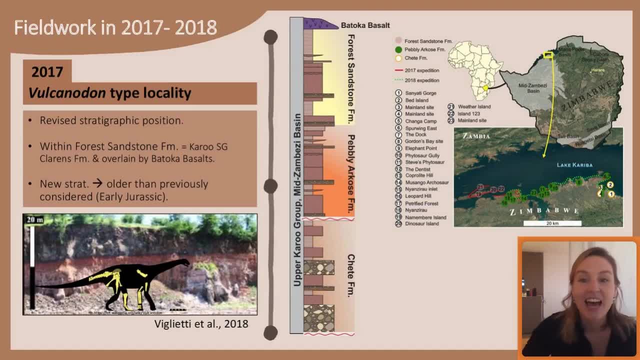 the southern shoreline of Lake Kariba and on several of the islands. One of the main aspects was to revisit Steve's collection and some of his sites, in addition to revisiting the type locality of Vulcanodon on Island 126-127,, and the results of which were: 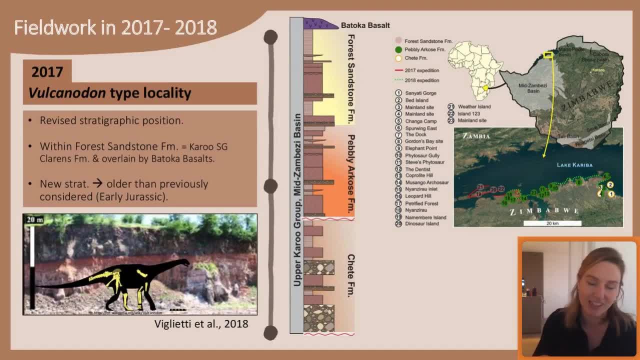 a revised stratigraphic position of Vulcanodon, making it all older than previously considered. And then, in 2018, we revisited several mainland sites and discovered several new fossiliferous localities, leading us to review and kind of refine the upper group stratigraphy within our 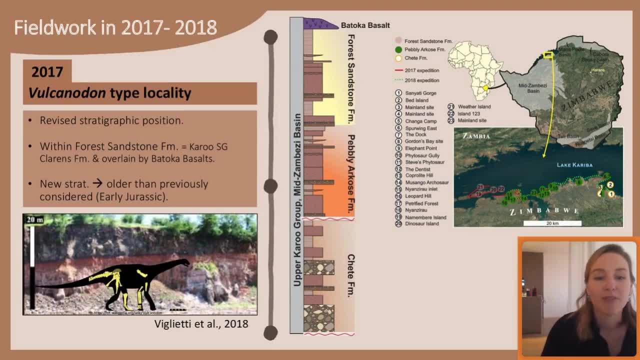 study area And that's where you can see that, in the middle of the slide, the log of the generalized stratigraphy. So we can now divide the upper Karoo group into three formations: the low-most Chete Formation, the middle Pebbly Arcos Formation and then the uppermost Forest Sandstone Formation. 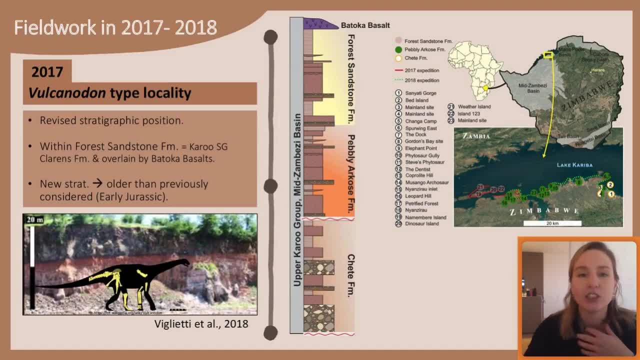 Which records sedimentation between roughly the middle late Triassic and into the early Jurassic. The Botoka basalts cap the sedimentary sequence and they are torsion age lavas genetically related to the Karoo-Large Igneous Province, Of particular interest to us in the fieldwork that we are. 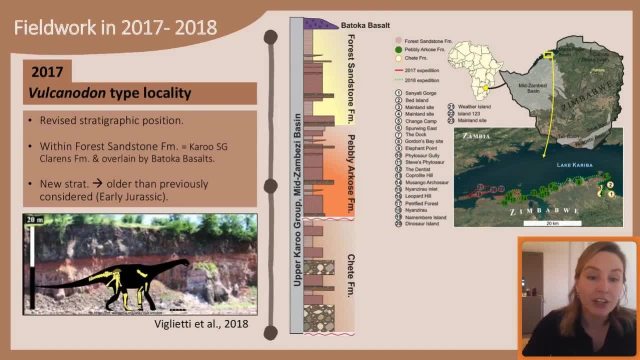 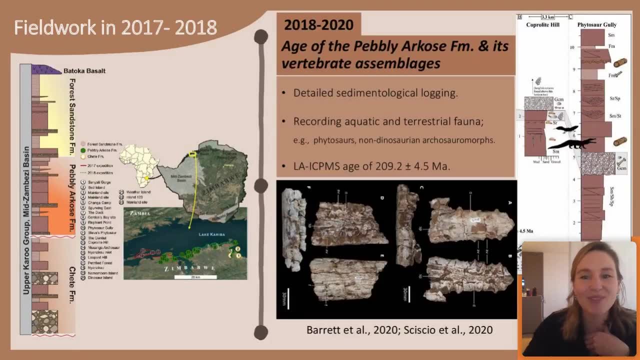 currently doing is the Pebbly Arcos Formation, previously only known to bear a bit of fossil wood and rare lungfish toothpaste in the Mitsambisi Basin. New slide, please: The Pebbly Arcos Formation. so between 2018 and 2020, we looked at the Pebbly Arcos Formation- has yielded a whole bunch of new. 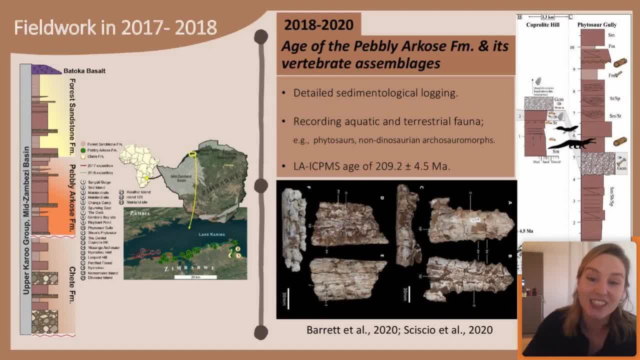 things previously unknown in sub-Saharan Africa, such as the phytosaurs which lay in credence to kind of late Triassic age for this particular formation. We also have the first detritial zircons from the upper Karoo group and from within the Pebbly Arcos Formation, giving it a maximum. 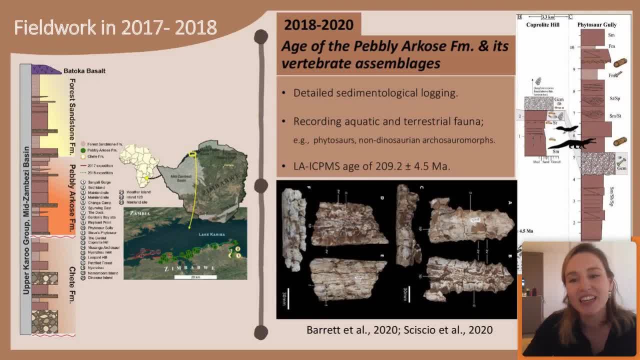 depositional age of about 209 million years, So roughly late, Nor-Early and recent in age, And this was the first time that we could have a more robust, concrete way of currently determining the age of the Pebbly Arcos Formation. So this is a very concrete way of correlating the upper Karoo. 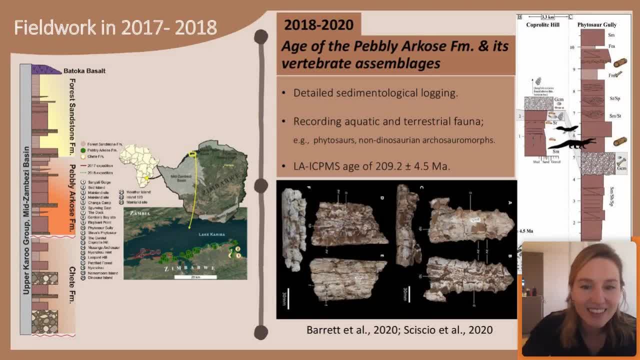 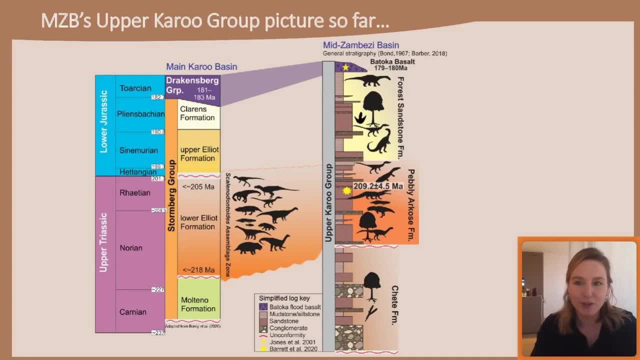 Group's Pebbly Arcos to the Stormberg Group in the main Karoo Basin. New slide please. New slide please. Thank you. So a developing picture of the upper Karoo Group so far in our little slice of the Mitsambisi Basin looks something like this on the far right You can. 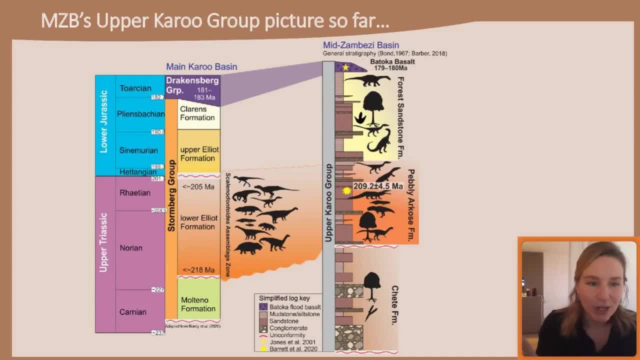 see that log and how it relates back to the main Karoo Basin on the left, And this is a work in progress but roughly. the Treti Formation is correlated with the Maltina Formation, based on a similar formation to the Maltina Formation. based on a similar formation to the Maltina Formation. 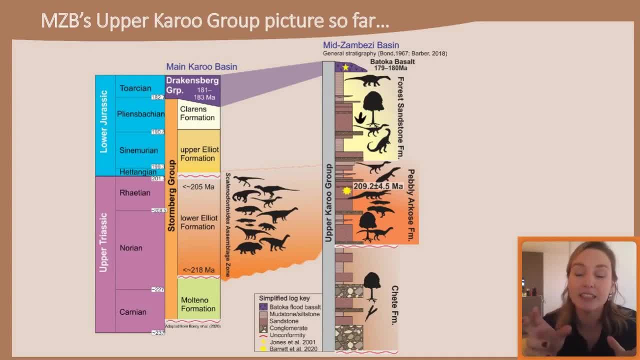 Our Pebbly Arcos Formation we can now say is more confident despite the lack of shared fauna, can be correlated to the Elliott Formation, specifically the lower Elliott, And then the Forest Sandstone can be correlated to the upper Elliott and Clarence Formations. 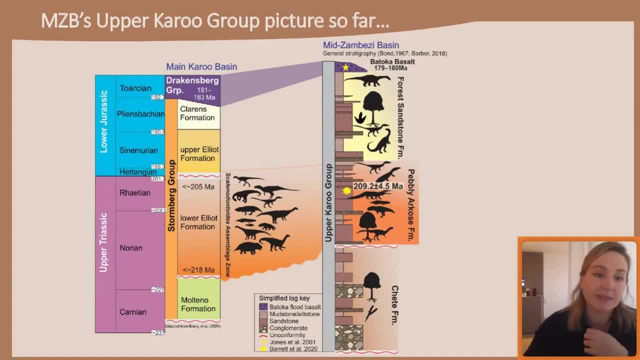 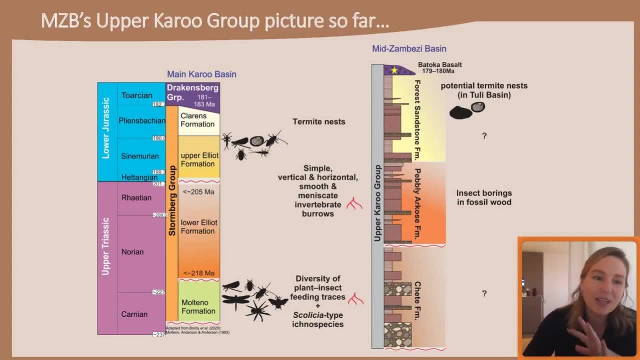 with those wonderful torsion lavas capping sedimentation in both basins. New slide please. But in terms of our invertebrate and plant body and trace fossils our picture is a little sparser for both basins In the main Karoo Basin, the Maltina Formation and one site in the upper. 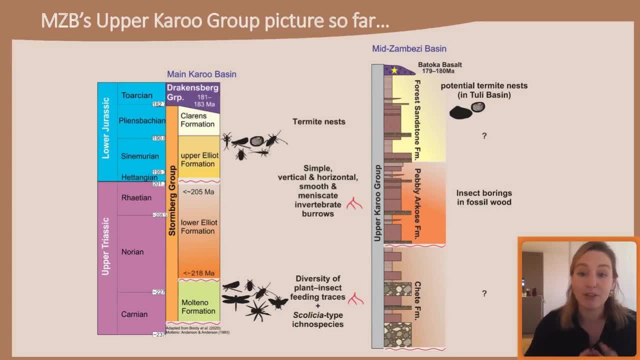 Elliott has a much more diverse insect and insect body fossil record including damselflies, dragonflies, cockroaches, gorilla, blactids and spiders. But the trace fossil record overall in the main Karoo Basin is quite limited so they have some simple invertebrate burrows and lack. 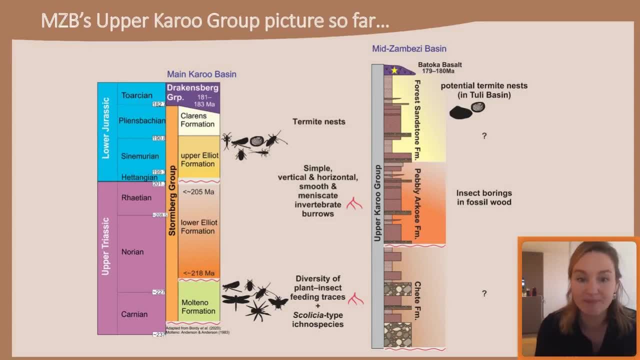 of detailed description or taxonomic assignment to most of those invertebrate traces. In our Mid-Zambesi Basin, where we've been working, it's even more dire and we only have one report of insect borings and fossil wood from the Pebbly Arcos Formation. Next slide, please. 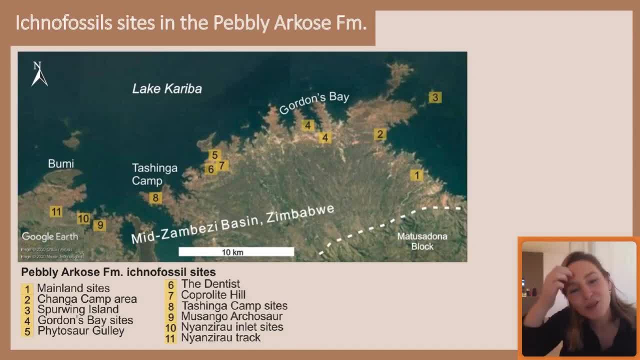 Next slide, please. With this in mind, during our fieldwork in the Pebbly Arcos Formation, we were recording, describing and logging any echno-fossil occurrences, and the map here shows the diversity of sites that we have that bear echno-fossils and undoubtedly this will be. 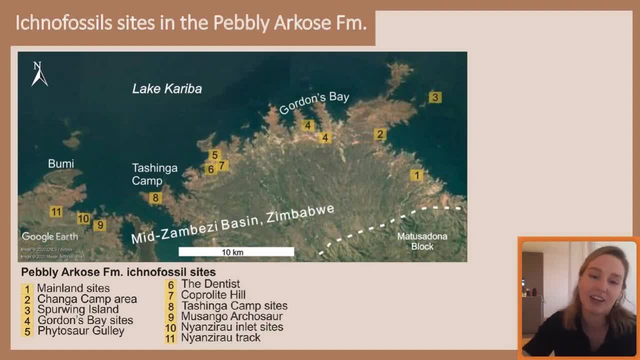 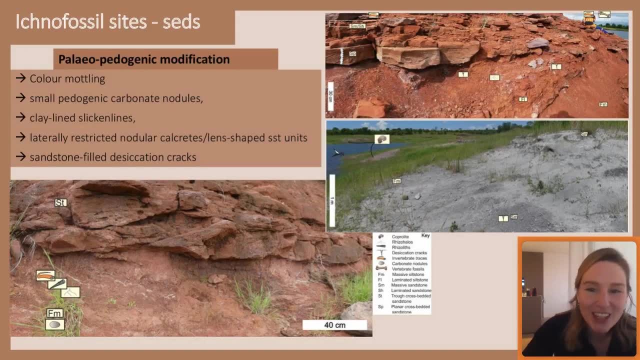 expanded within the Pebbly Arcos Formation and probably into the underlying and overlying formations. with more exploration, Next slide, please. Okay, so from a sedimentological perspective, the Pebbly Arcos Formation represents a Fluvio lacustrine redbed. 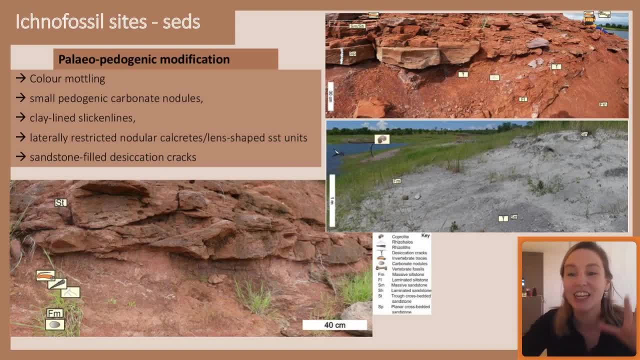 Next slide, please. Next slide, please. That can be really roughly broadly divided into channel and floodplain fine elements and our echno-fossil bearing sites. the trace fossil bearing sites were documented mainly in those floodbank finds for overbank areas, and these can then further be subdivided based on. 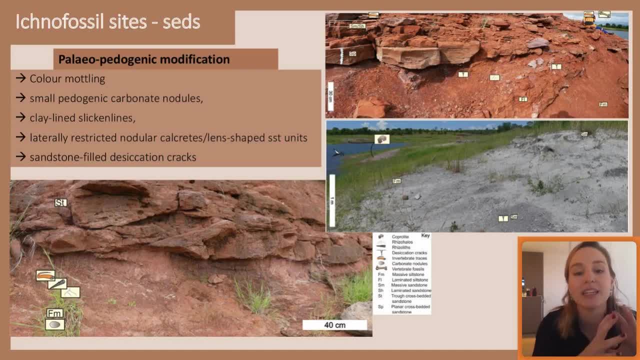 the degree of paleopetigenesis that these sites recorded. So we have some sites that are strongly developed, paleopetigenic features, such as the site on the far left at bottom corner, which has been downcut by some trough cross-bedded sandstones, and then we have more weakly. 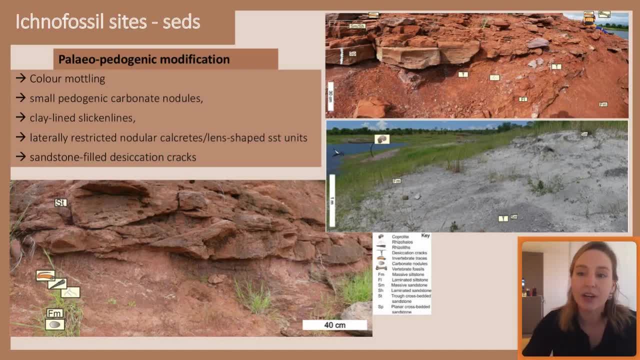 paleopetigenically modified profiles which have more interlayering of laterally discontinuous sheet and lens shaped sandstones indicating some short, punctuated high energy events, such as crevice, blaze and fluvial channels cross-cutting the floodplain. 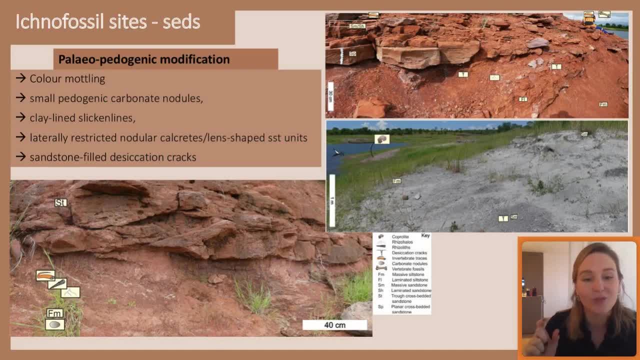 And often we see in those sites echno-fossils that are really taking advantage of those short-lived, ephemeral events which are bringing nutrients onto the floodplain. Next slide, please, Next slide, please, Next slide, please. 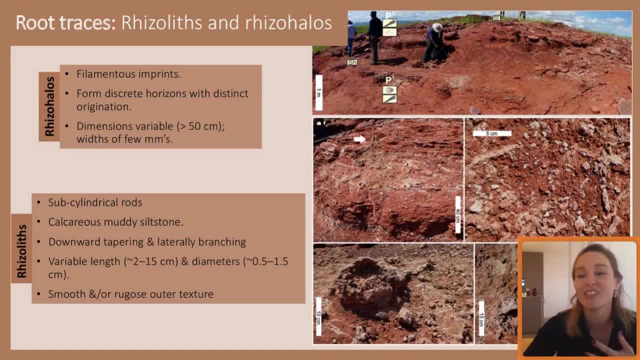 root traces. so, in terms of our plant trace fossils, we have rhizohalos and calcareous rhizolus. these are quite common at all of our sites, but mainly in the strongly paleopetrogenically modified sites. of interest to us were the rhizolus, which were always calcareous. they're sub-cylindrical rods. 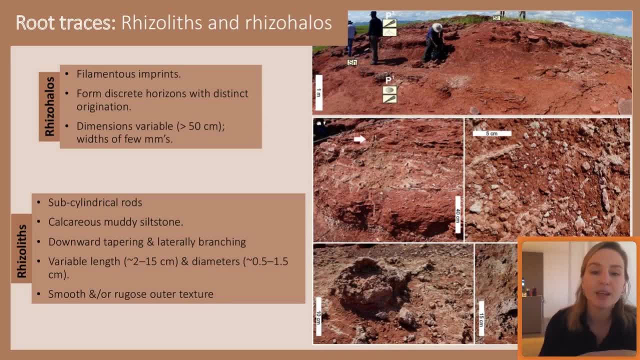 composed of very fine-grained sandstone and carbonate. we had some- uniquely, some larger calcareous rhizolus that were about 10 to 20 centimeters in diameter perpendicular to the bedding and that can be seen in the middle left-hand photograph and the one directly 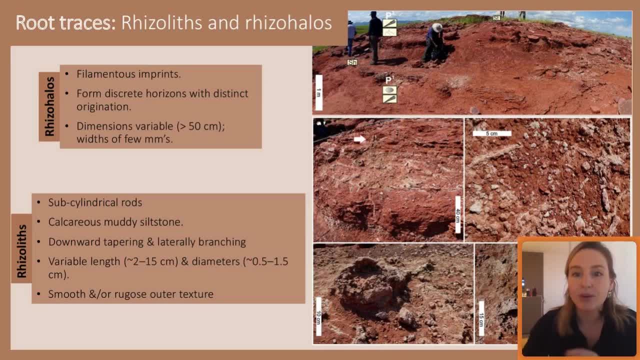 below it with the white arrow and these um often sometimes showed smaller calcareous rhizolus and peter tubules. that kind of radio radiated away from that central column. in some cases the calcareous rhizolus at our paleo um paleo souls completely obliterated any of the bedding that. 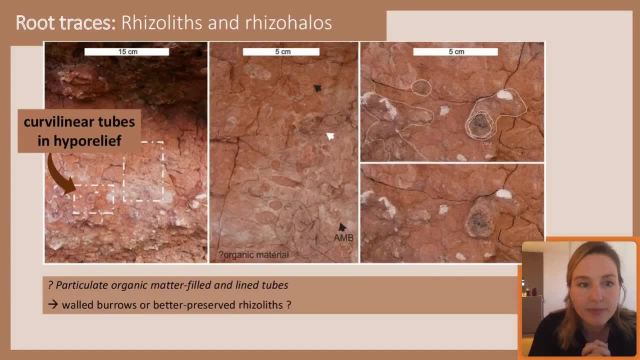 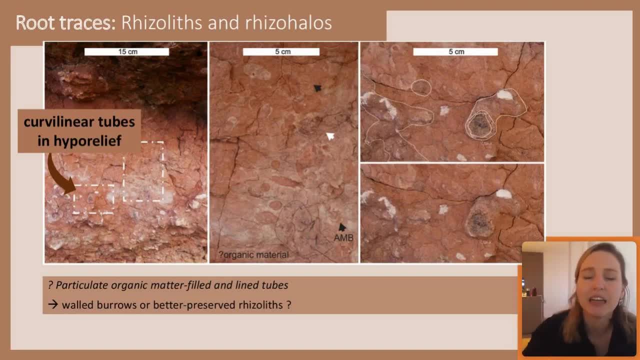 and uniquely, we also saw these organic uh matter filled and lined tubes. they're about two to four centimeters in length and they're shown on the very far right, and they're walled between one and two millimeter thick walls with a total diameter of approximately two centimeters. the walls were 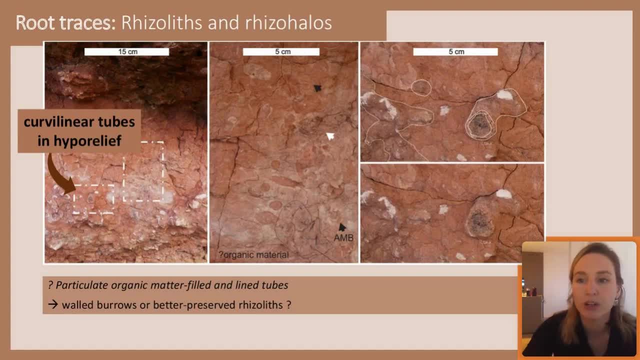 made up of silty, very fine-grained sandstone, whereas the infill is composed of more muddy siltstone, and what was so unique is that they seem to be filled with particulate dark material matter, less than a millimeter in size, quite soft and conspicuous throughout the matrix, but more 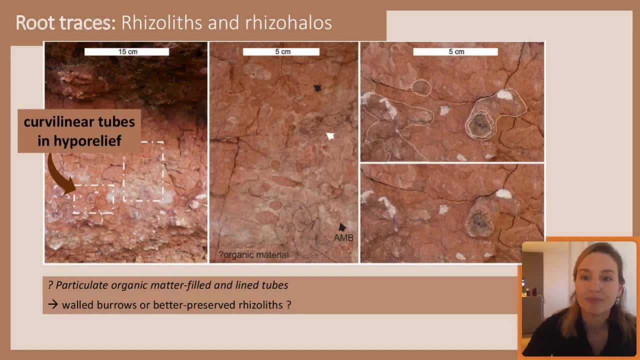 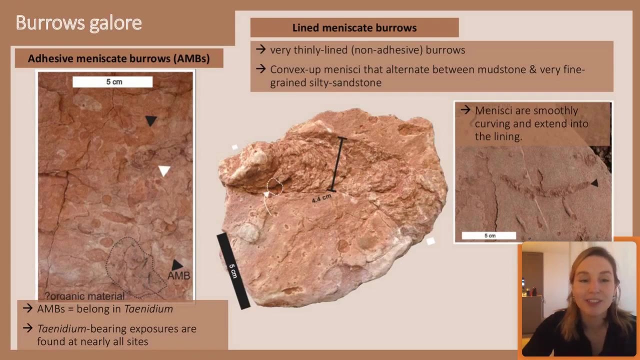 marginally um concentrate, concentrated within the infill. it's unclear if these were wall burrows in this section or better preserved rhizolus. so something unusual in that paleo soul. next slide, please. moving on to the invertebrates burrows, so we have several sites bearing invertebrates, most 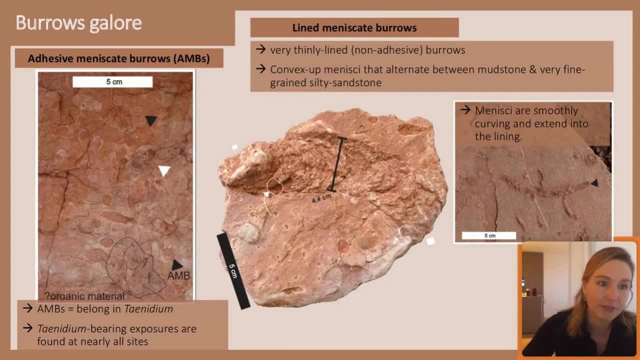 copious with the meniscus burrows, so i'm going to deal with very far left adhesive meniscus burrows. these develop as distinctly alternating: maroon to pink, pale pink menisci of the same material and straight to curvy, curvy, linear burrows. the adhesive meniscus burrows can be described as: 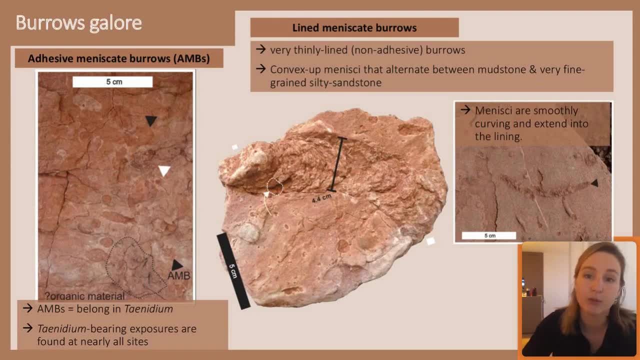 to medium and we saw these in most of our sites that were really strongly pedogenically modified. in the middle of the slide we see another meniscus burrow. this is one of the much larger meniscus burrows. it was four to five centimeters in diameter and, importantly, it 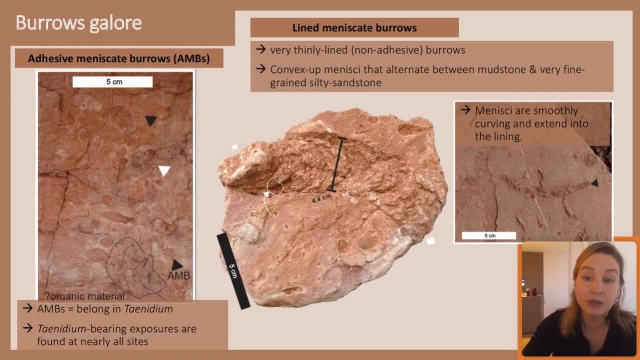 is lined, or it had it. it had a thin wall, the meniscus two were alternating between red mud stone and a lighter pink, calcretized sort of very fine grained silty sandstone, and they were. these burrows were prominent in weakly developed paleo souls and in association with in situ. 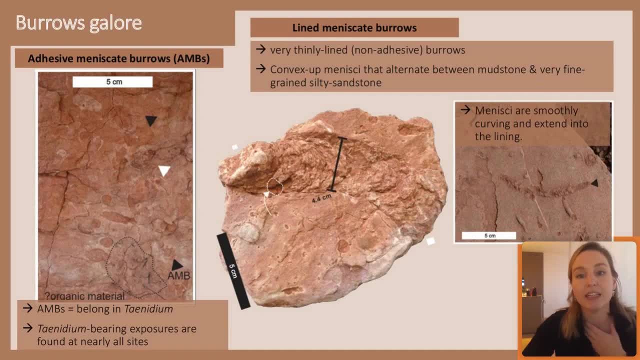 vertebrate material. then on the very far right of that slide we see um another type of meniscus burrows. so these are much smaller. so between seven millimeters and a centimeter in diameter they're lined again, and with meniscus and a heterogeneous alternating meniscus of 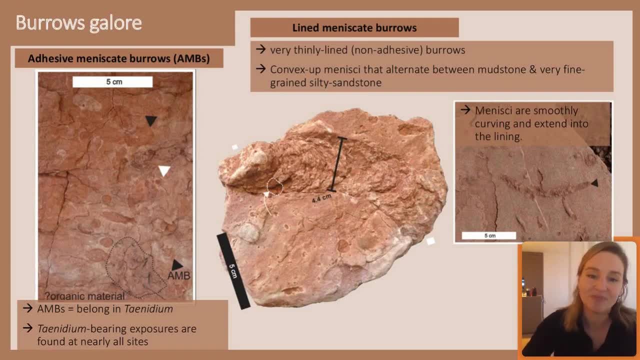 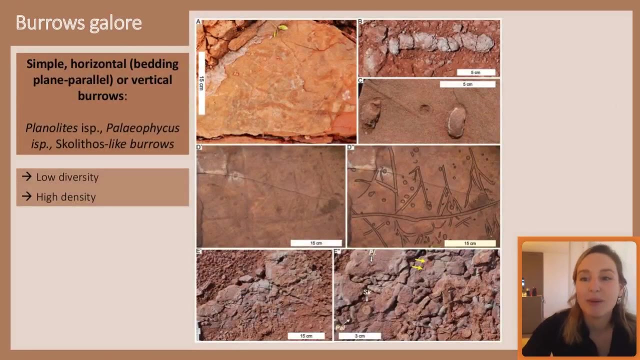 different materials, again of very fine sandstone with mudstone. in these traces the meniscus are are smoothly curving and can be seen to extend into the lining um and these burrows sort of resemble anchoriness um. next slide, please. other commonly noted burrows within the pebbly archos. 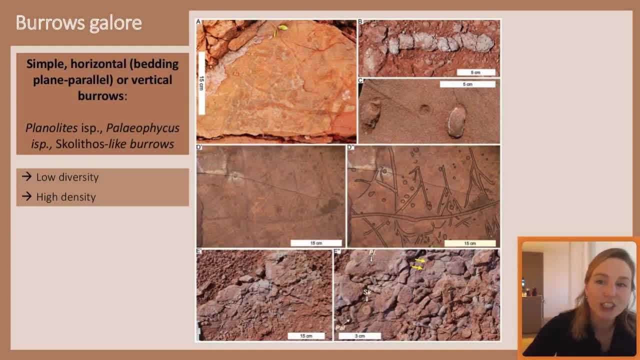 formation are simple: horizontal, straight to slightly curving, non-branching forms with no wall or lining, really simple forms that can be referable to planolites, and the top two pictures illustrate those burrows and then similar to planolites but showing a very thin lining. we 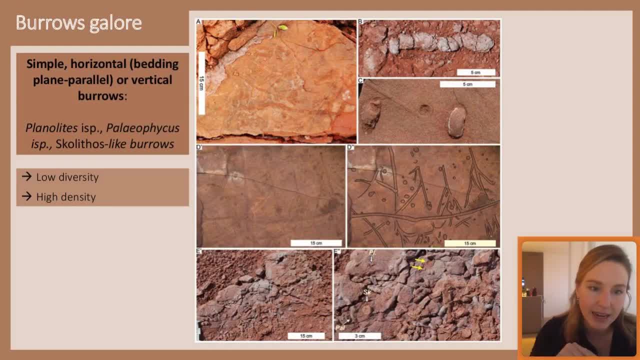 also had paleophycus, which are represented in the bottom photos under the acronym pal, and at several sites we also had vertical bedding plane perpendicular burrows in association with the planolites and paleophycus like burrows which could be referred to as either skeletal- certainly skeletal like- and then we also see a variety of 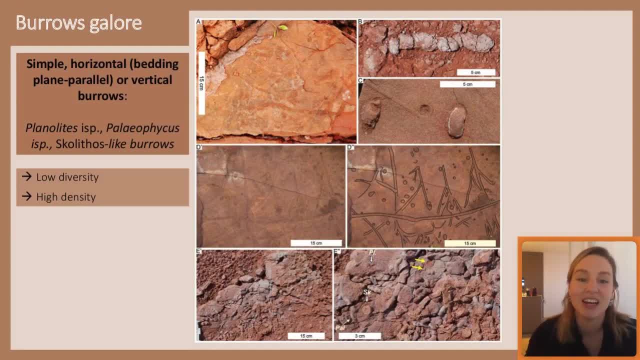 forms that are not placed into any specific echnogenes but can be described um but could be described. so we in the middle there and the um, we have these unique y-shaped branch burrows that are buried in plain parallel and overall what we're seeing with the traces. they're generally 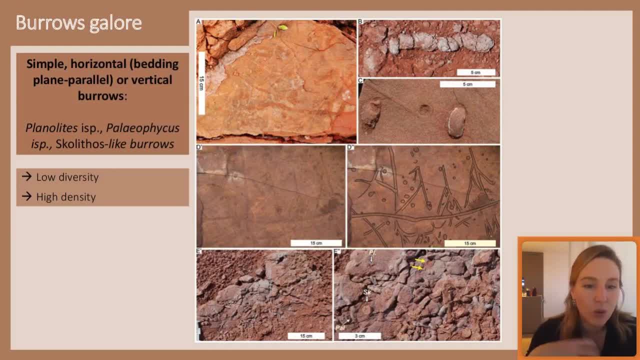 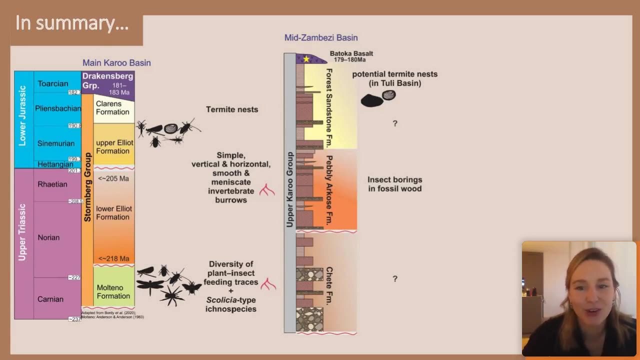 represent quite a low diversity of uniforms, but um are always in quite high density on the surfaces or in the sedimentary units that they're found. next slide, please. so, in summary, our previous understanding of the upper crew group, and specifically pebbly archos, in terms of invertebrate. 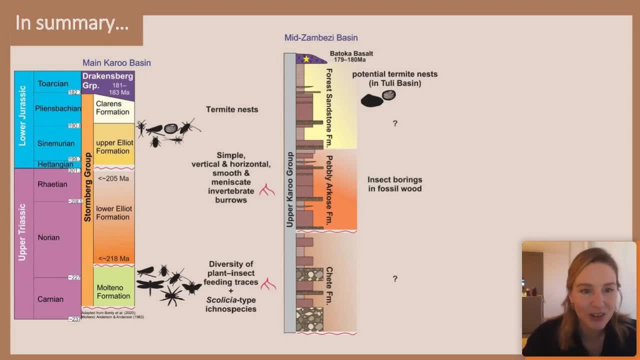 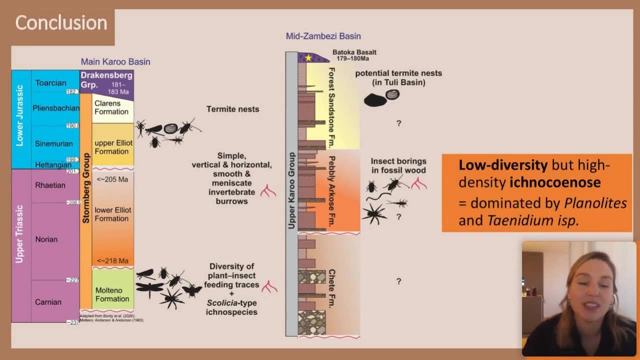 plant and plant trace fossils is quite sparse. we don't know a hell of a lot and there's much to be explored. next slide, please, but now we're building a bigger picture. so invertebrate echno fossils probably represent quite a low diversity but generally quite a high density of different traces that are. 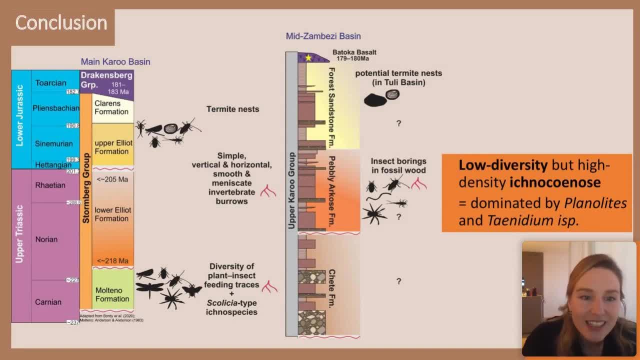 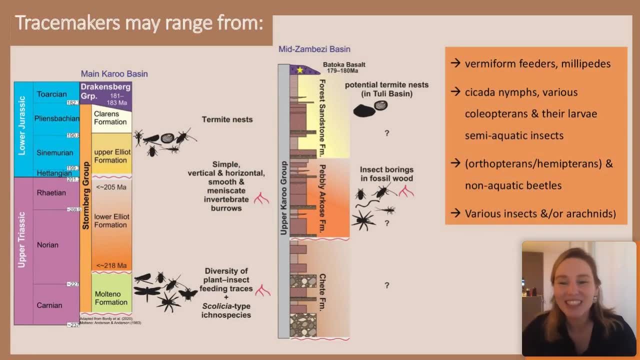 typically dominated by planolites and tanadium. next slide. please thank you. um. tracemakers, which have been typically attributed to these echno fossils, can range from orthopterans to coloptrons in their lava and vermiform feeders, and millipedes um. next slide. 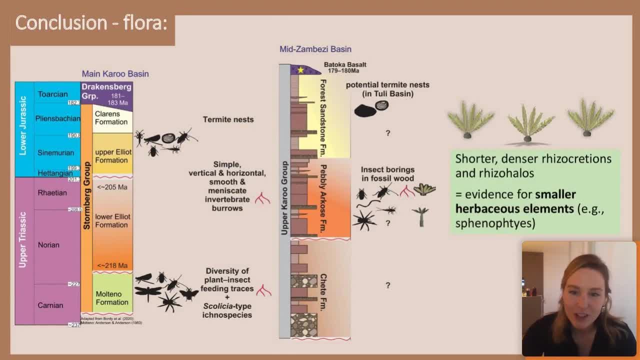 please. and in terms of our plant trace fossils, um largely they're represented by those um short interconnected calcareous rhizolus that can be likened to fibrous root systems typical of today's monocots and ferns, and while we only have fossil wood in the pebbly archos formation relating to 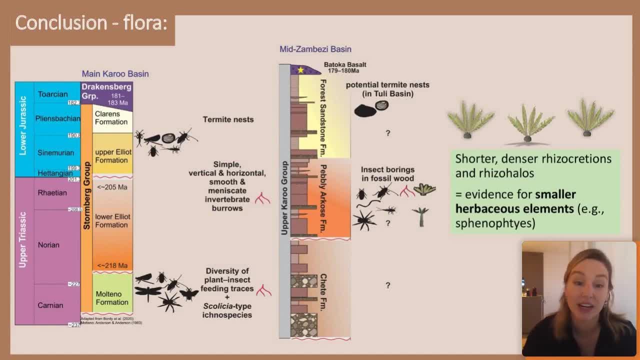 some sort of conifer family such as didaxalon. we don't record any other flores in the pebbly archos. however, in the underlying cheta formation we have a presence, we have the presence of diacridium floral assemblages and it could be expected, or 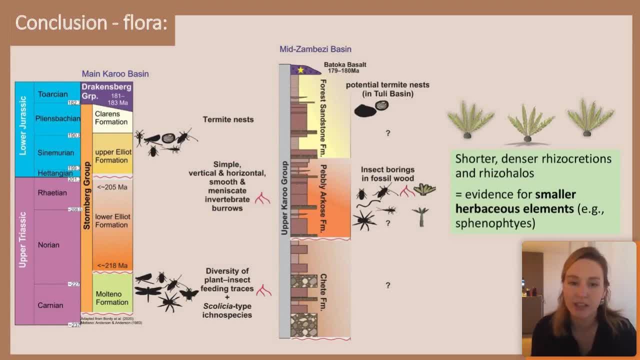 we might expect that you could see similar herbaceous shrubs, horsetails and the likes that we see in the underlying formation, creating the diversity of root traces that we see in the pebbly archos formation and all together, um, in summary, the we have these echno fossils. they're making 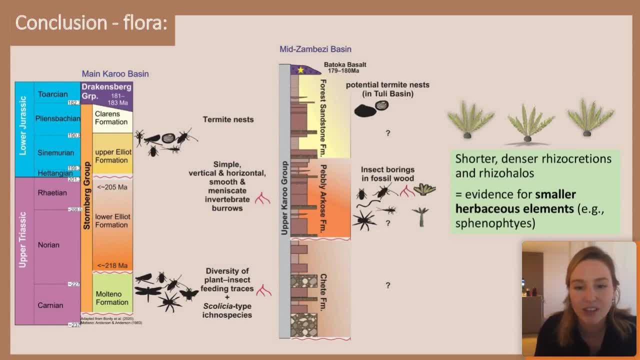 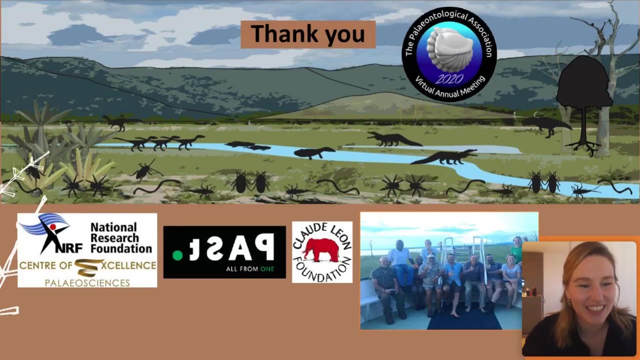 inroads and into and broadening our understanding of the pebbly archos, late trisic overbank areas, in addition to um expanding the potential ecosystems that we're seeing and complementing our currently known and expanding aquatic and terrestrial fauna. next slide, please, and thank you very much. sorry about the technical. 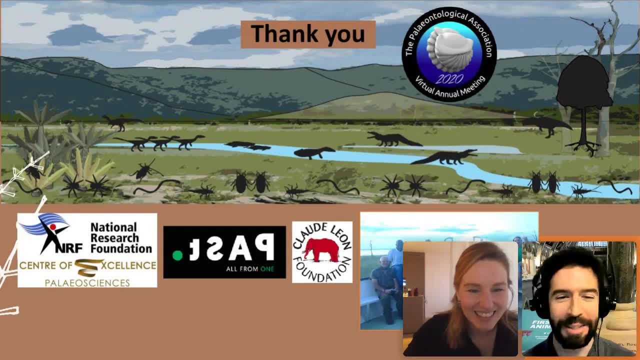 flip? not at all. i actually i gave you one minute to give thanks. i like that. that was a very nice thing to do, all right, so thanks so much for your, for your, for your talk, uh, and i believe we have uh one question here in chat. please do feel free to drop questions for. 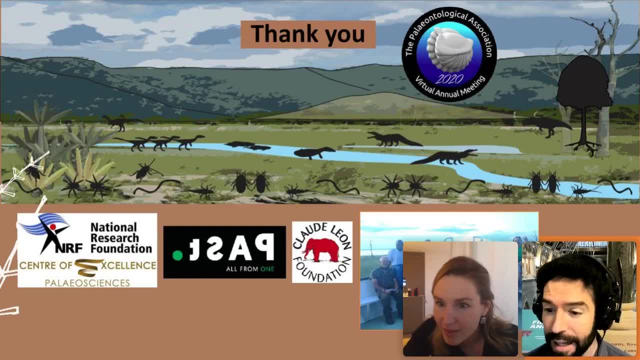 um for lara in the in the chat and here one for you that says: let's see, you show that. did you show that the forest sandstone occurs in the appliance vacuum and do you see any evidence for increased continental aridity in this time period? okay, so to answer that sort of in a nutshell, we do. overall, there is increasing aridity. same as what? 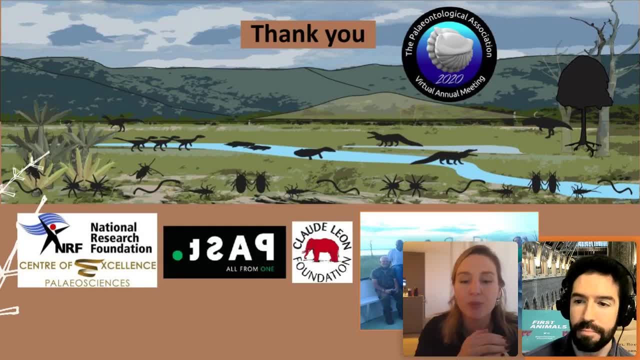 is seen in the main crew basin. so we'll try to answer a little bit in this video as well and we'll, within the upper crew group you're seeing sort of braided going into meandering fluvial systems and then in the forest sensor, in particular the lowermost part of the forest sandstone you're. 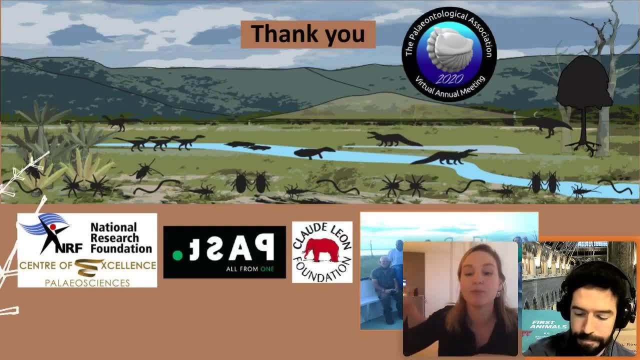 seeing more um fluvial action and then the upper part. you see more alien conditions being generated and it's in that uppermost part where the volcanodon was discovered in, i think, a fluvial interbed, but within a broader context of being in your alien depositional environment and the age. 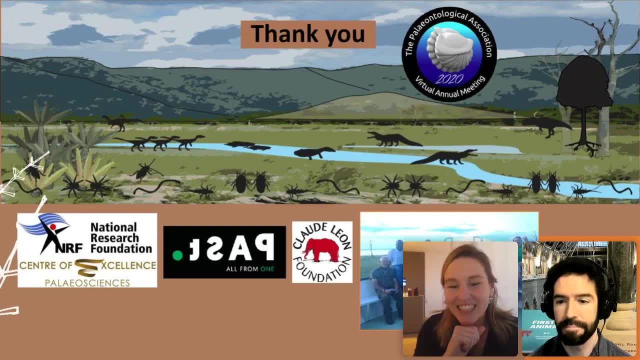 for the, the forest sandstone. it's a really good question, um. that's something we're still working on. i think it might have quite a large spread or always seeing lots of um unconformities within that formation. definitely, it probably is, at least in part, conspiring nice. another question for you. 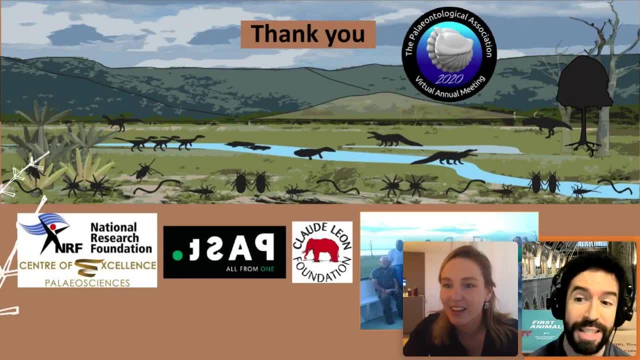 here. can we, can you be certain that the invertebrate trace assemblages are ignocinosis and therefore produced right by fauna living in the same place at the same time, rather than printing of traces from different communities? i think in some regards, in some of the sections, 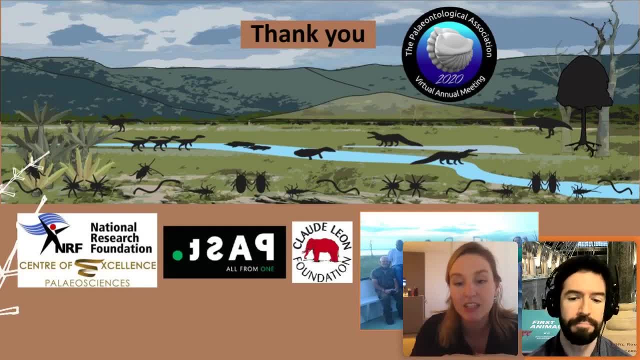 that we see we have a distinct overlapping of traces that appear at the same time, and then we have over printing by later- um with how late, i'm not sure, but at least late enough- where the first set of fauna, uh igno fauna, have been solidified enough to then be, secondarily, uh, 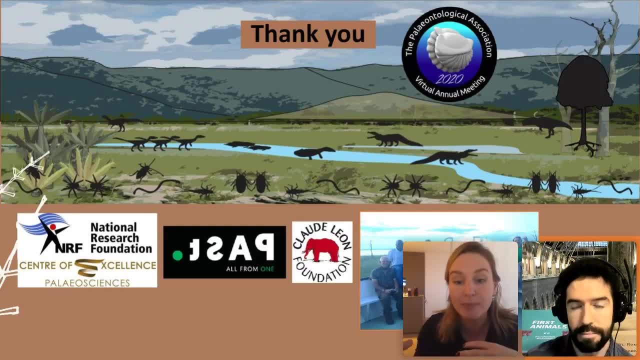 bioturbated by later animals. so we do see sometimes two assemblages stacked on top of one another. um, i've lost my train of thought, but i think, yeah, we do at least have one grouping of animals that we see and and we know that then we get a secondary um later bioturbation of that first set. 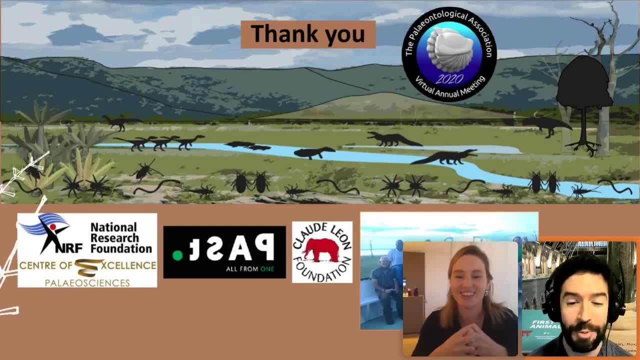 all right. thanks so much, martha, and we'll now move on to our next speaker. feel free again to drop questions, for i'm sorry, i'm calling you martha all the time. lara, cool, thank you very much. so many numbers. feel free to drop questions for lara. 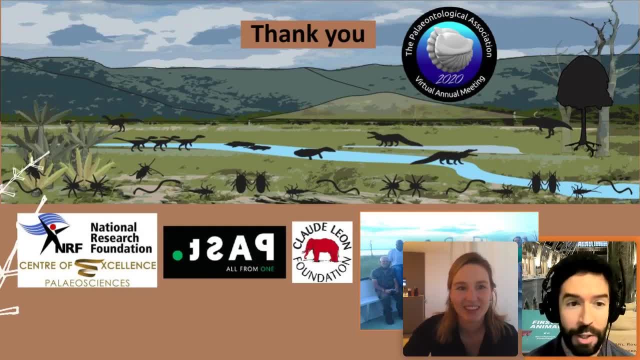 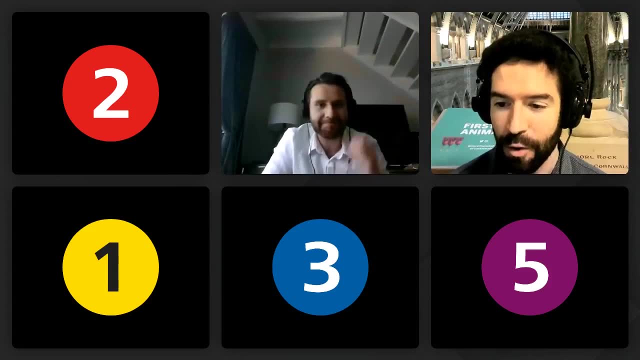 in the in the chat. um, okay, now we'll move on to the next speaker. uh, cameron, are you over there diving clear? all right, so hopefully i will not call you martha, although you know i i would not rule out that. sorry about that. alright, so your talk is here and it's all yours. 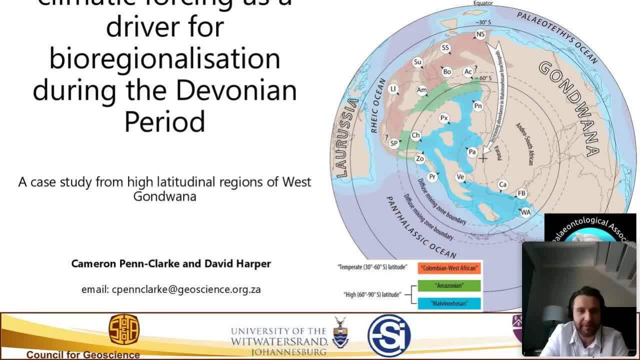 thanks. thank you very much. the introduction and welcome everyone. uh, today's talk i'm giving is on research that I'm doing in conjunction with the Council for Geoscience, Wits University and Durham University, looking at high latitude change during the Devonian. but this talk 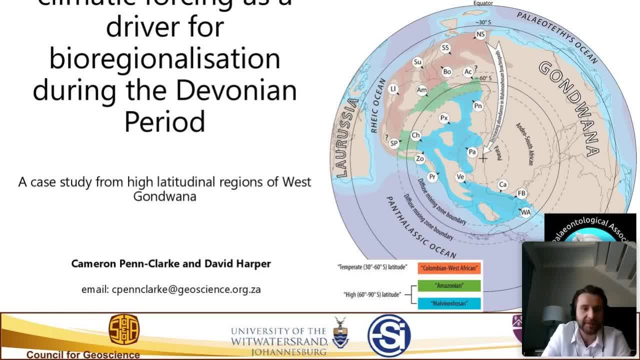 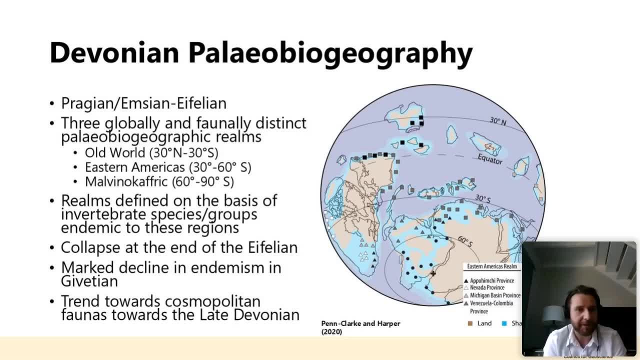 for today is focusing on bioregionalization. So during the Devonian period between the Praguian Emsian until the Athelian, so latest early Devonian to earliest middle Devonian, you saw unmasked bioregional development of bioregional provinces or realms throughout. 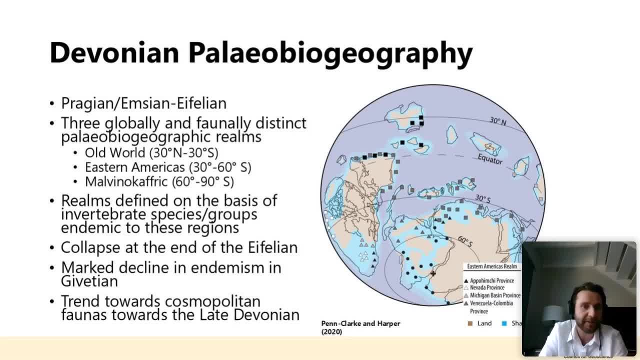 the world. These could be divided into the Old World, Eastern Americas and the Malvino Capric, And these are defined on the basis of several endemic invertebrate groups. And towards the end of the Athelian, you see a complete collapse in this entirely. And then 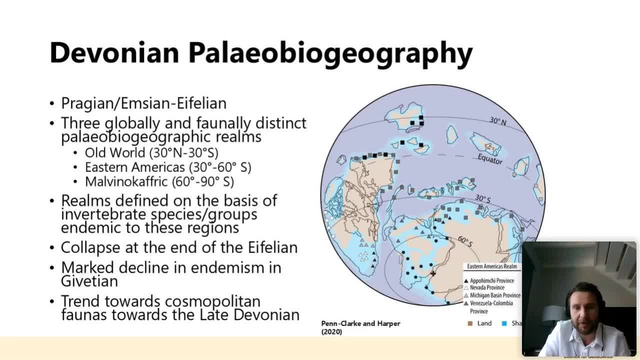 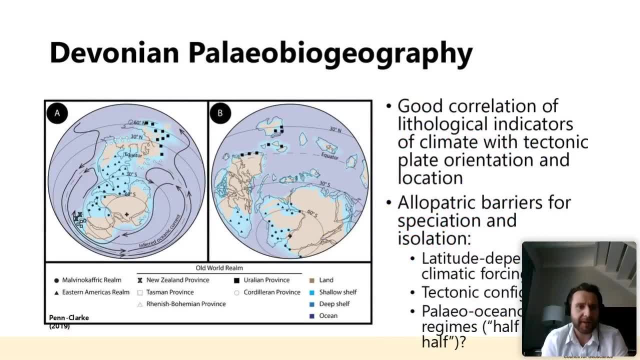 moving into the Jvertian and into the late devonian, you see more cosmopolitan foreigners taking appearing globally. so, uh, it does appear as if these uh broad bioregions were constrained in latitudinal bands. um, so this has got people thinking. as well as that, um, was this latitude dependent climatic? 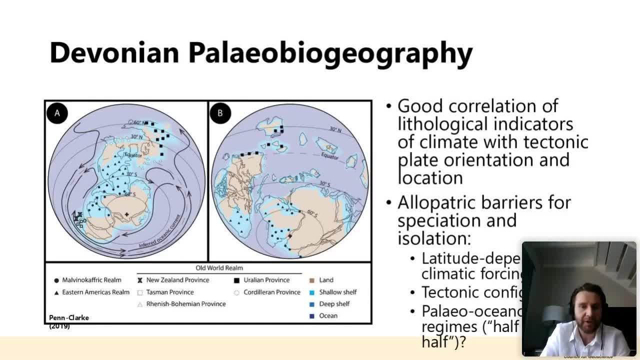 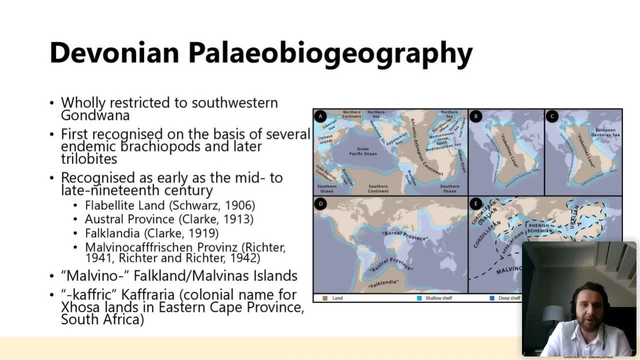 forcing? was it something to the tectonic configurations or paleo oceanographic regimes? um, so, could it. could these have acted as allopatric barriers for speciation and isolation? uh, so, moving on to the high latitudes, um, we were uh considered high latitudes, the malvino. 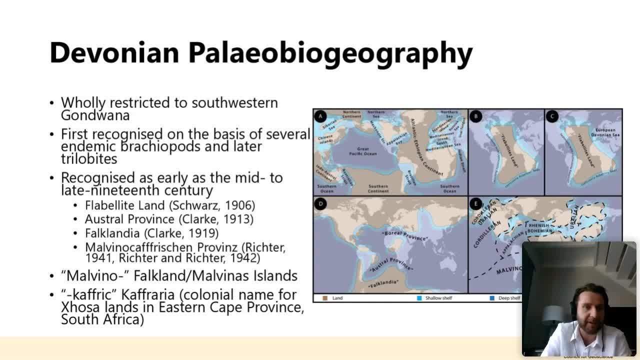 capricorn, so this was completely restricted. southwestern gondwana, and this was first recognized on the basis of several endemic brachiopods and later trilobites that went through a bunch of different names. first there's flavolite land, the austral province, forlandia, the malvino, 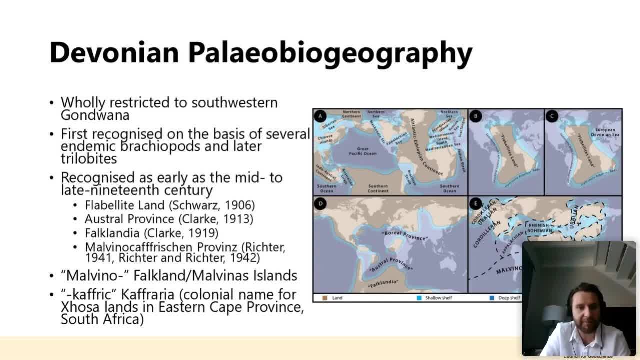 caphrasian province came later in the the mid-20th century uh, by the richters, and so the etymology of it, of course, is derived from malvino, from the falkland or malvinas islands, depending uh on your persuasion, and then kafric, from kafraria, which is the old colonial name for 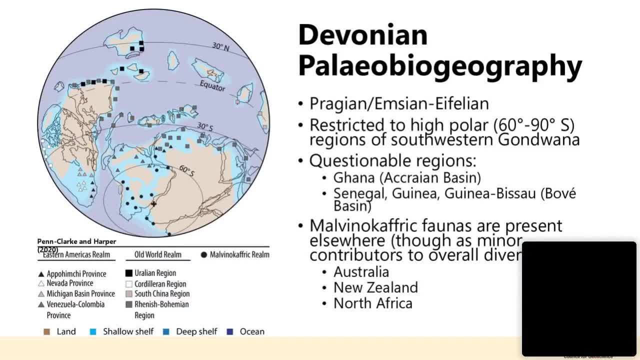 the most of the names in the eastern cape province of south africa. um, so we? um, yeah, this, the malvino capric rome seemed to have been also restricted to these highest latitudes. questionable areas that were included. so ghana, senegal, guinea, guinea-guessau? um, we're not really sure if they fit. 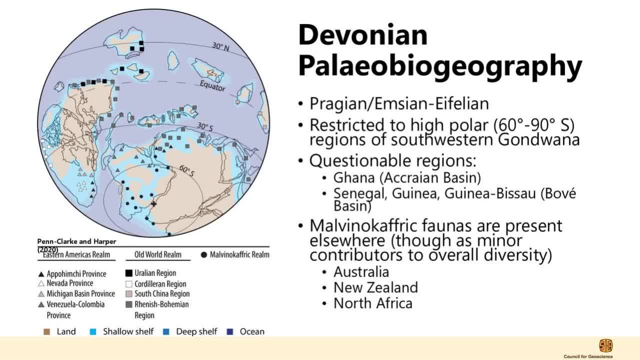 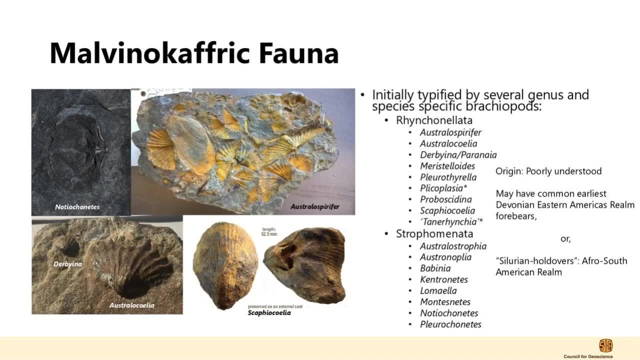 in there because we do find malvino capric taxa, but there are foreigners elsewhere in australia- new rica, so one or two little guys that you know just escaped these polar regions. so there's a bunch of endemic taxa over here. uh, the the main indicator taxa of australia, spiropha, australia, celia. 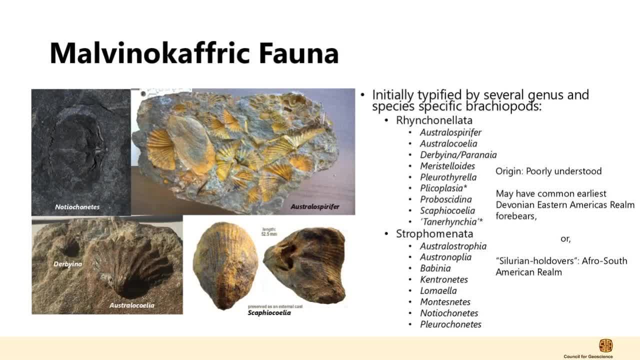 lubina and pleurothyrella, australostrophia and pleurokinetes notokinetes in terms of brachiopods. so we we think that these came from having an earliest devonian eastern american realm originator, or they could be silurian holdovers from the afro-south american realm. you're not really sure. 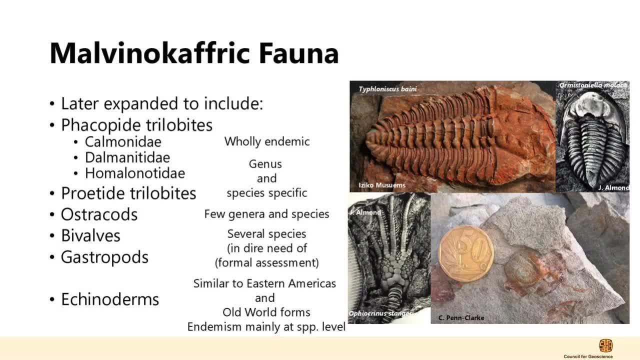 uh, trilobites. there are a bunch of the coped or back apart um trilobites that are endemic. so the calm monads, the entire group, is um endemic. they're mantids homologated, some proteids, ostracods um, and then bibles, gastropods in the kind of rooms you're not really sure what. 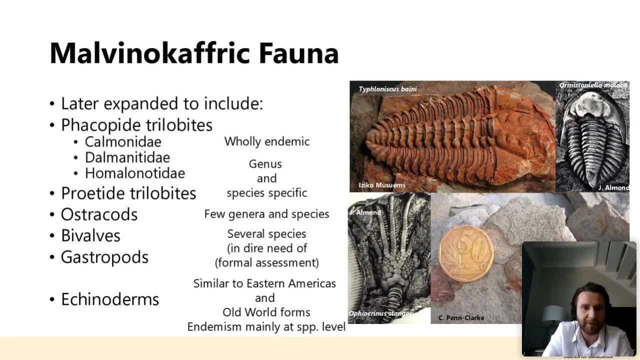 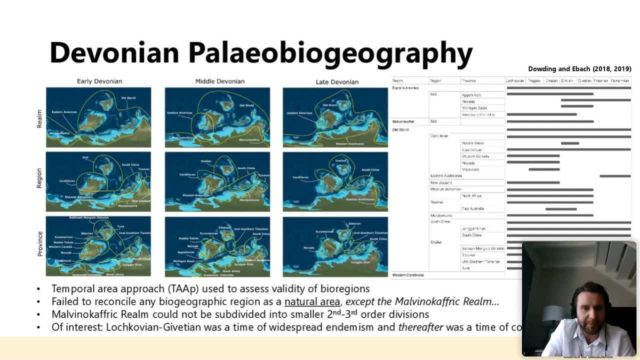 endemism looks like there, but they do seem to be very um, cosmopolitan. previously killings, yep, all they are. aqu Thing is gonna needed to be declared. so uh, preface studies were. more recent studies took a looked at the validity of these bioregions and, um, these showed that all of that, none of these biogeographic regions, 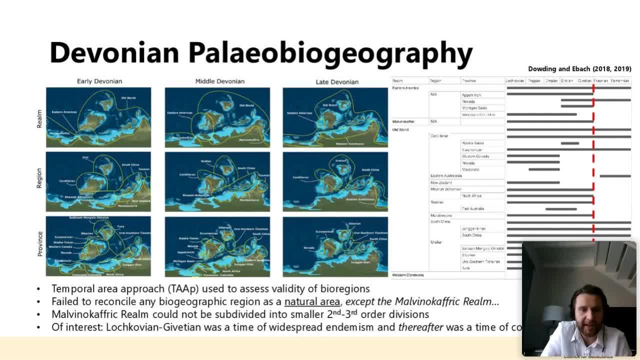 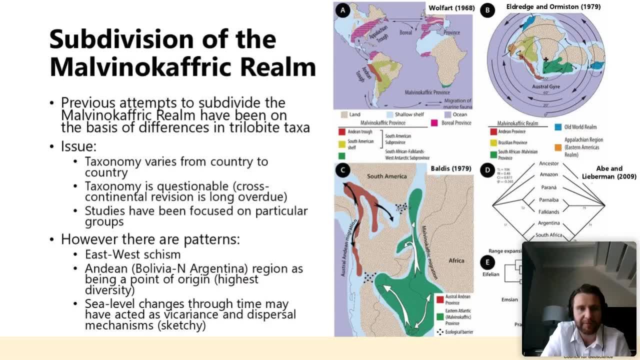 uh, are real, um, except for the malve Throw, but they cannot. we could not divide these further. and of interest is that, wherever you look globally, the lakovian javadian was a time of widespread endemism and thereafter cosmopolitanism. uh, previous attempts to try and subdivide the mauritianism on all. 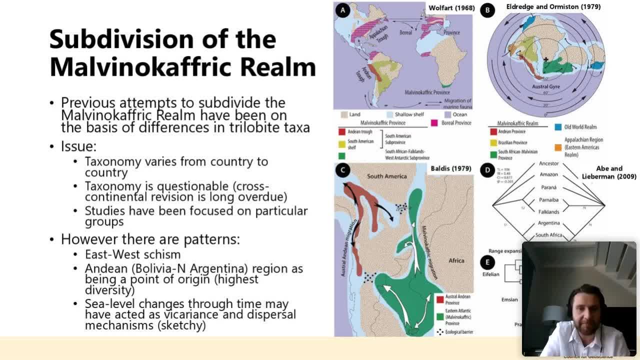 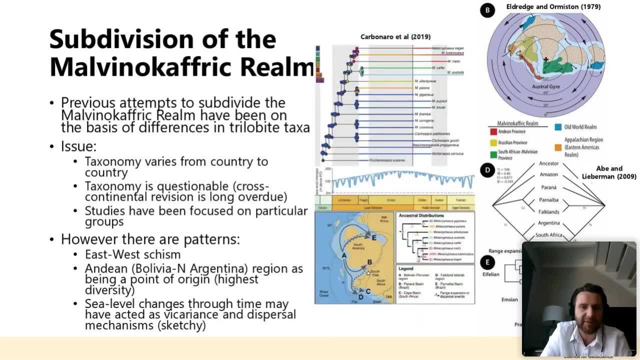 try and subdivide the Malvino, Capri, Grom have have taken place in the past using trilobites, but there's, you know, there doesn't seem to be any agreement, and this is because taxonomy is quite poor. but one thing we do see is an east-west schism of a Andean center where, with the highest, 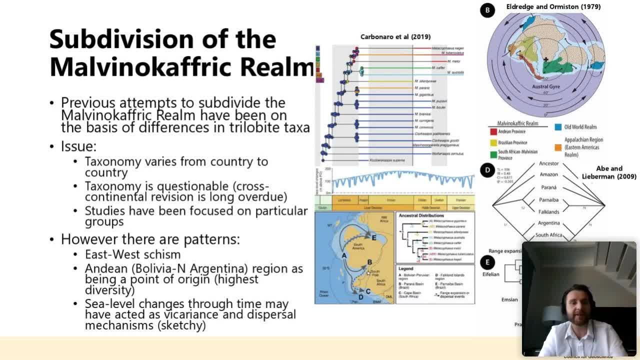 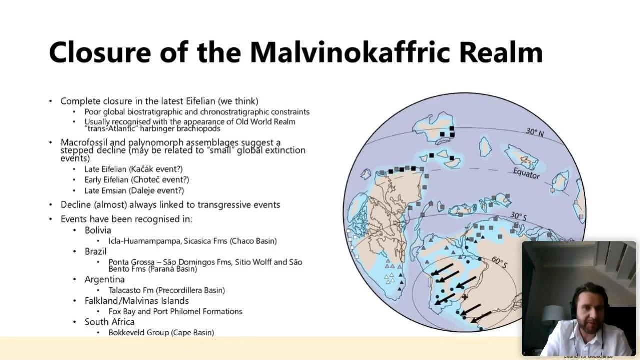 points of diversity and a eastern part with lesser diversity. so previous studies have thought that sea level acted as a vicarious and dispersal mechanisms. but again, if you believe in global sea level curves being real things, that's to be debated. so the closure of the Malvino Capri Grom. 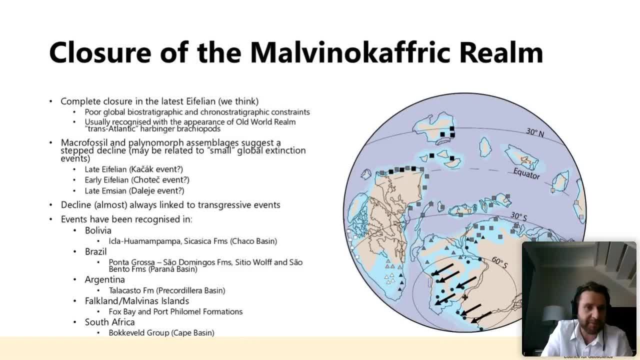 seems like it could have occurred with several extinction events coincided: the Katschak, the Shottesh, the Dalesh events. we're not really sure because timing constraints are quite poor, but the decline always seems to be linked to transgressive events and it's been recognized. 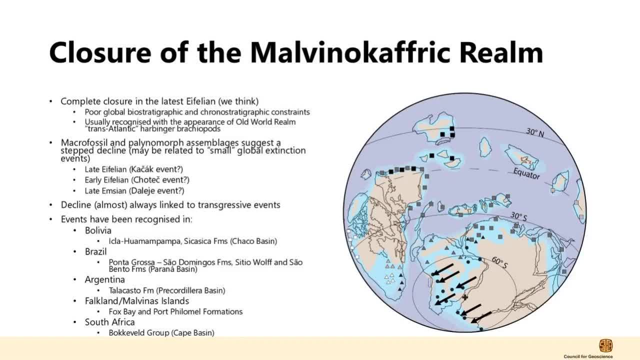 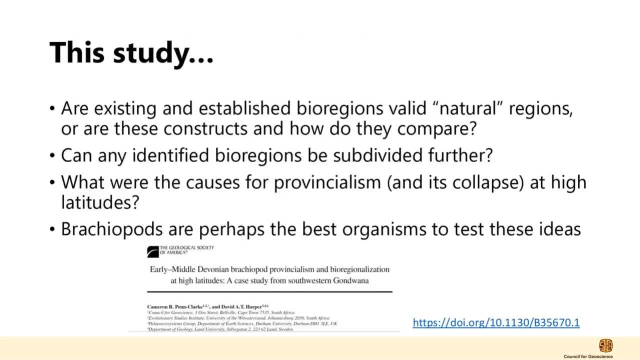 now over most of southwestern Gondwana and generally when, when you have these harbinger old world ground brachiopods, generally the appearance of Rapido thyrus or Tropida leptis in large quantities normally end or normally signals at the end of the Malvino Capri Grom. 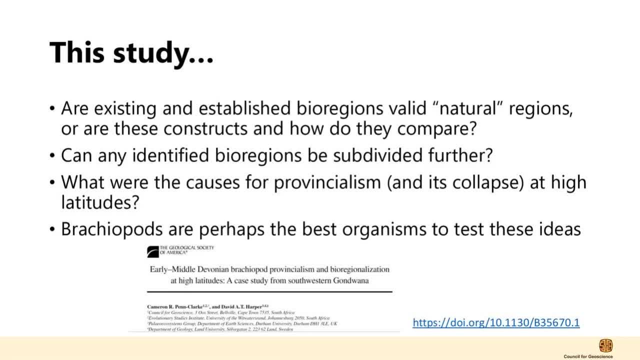 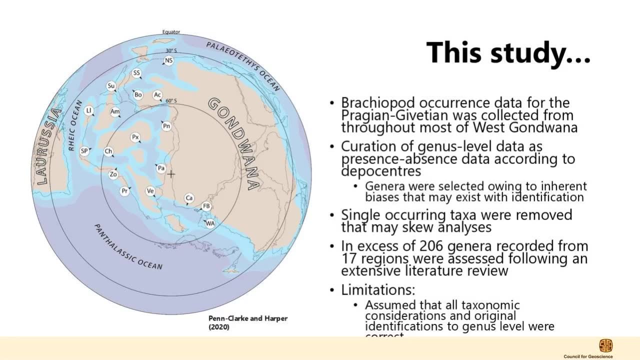 so, walking into our study now, we looked, we tried to see if any of these bioregions are natural bioregions. can they be subdivided further? what were the causes for provincialism? and we looked at brachiopods in particular. so we managed to amass a huge data set comprising over 206 genera. 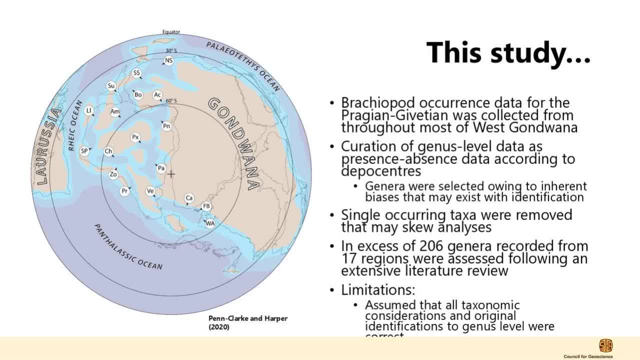 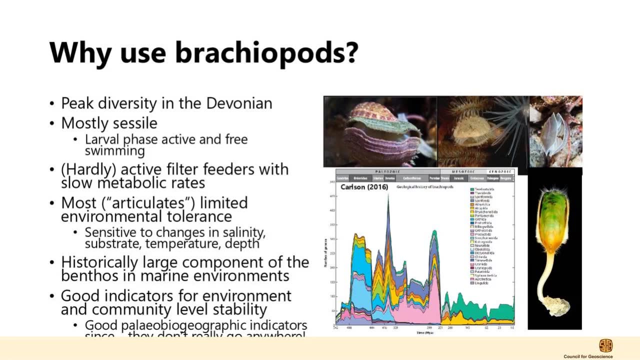 from 17 regions around southwestern Gondwana. but this study is limited in that we can we assume that all taxonomic considerations and original ids, down to genus level at least, were correct. so why use brachiopods? they don't really do much, so they are filter feeders. they're very good. 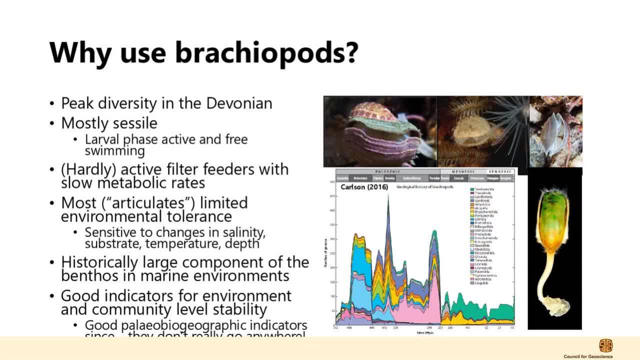 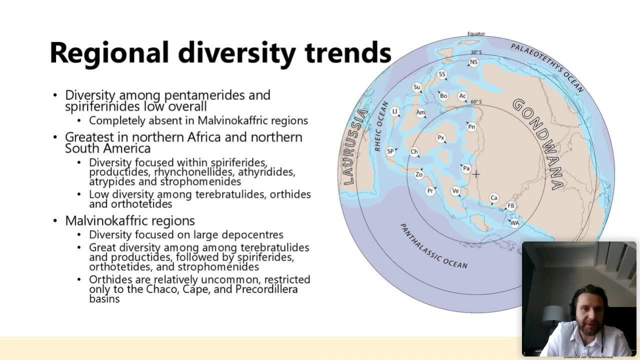 indicators of benthonic environments and health because they don't move anywhere. so, yeah, that's why we decided to use them, because they would be very sensitive to changes of salinity, substrate, temperature and depth. so the regional trends that we did observe is that pantamorides and sporiphanides 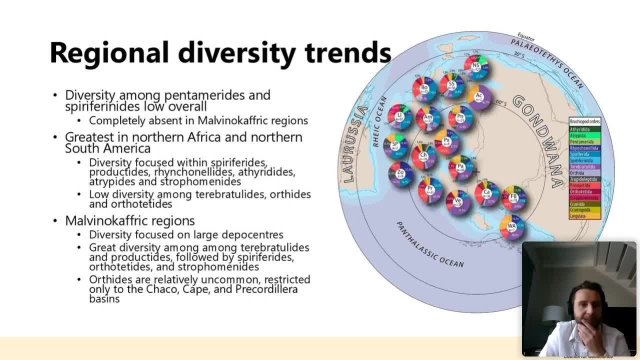 are missing, so they're not important in the study, but they do have a very high tourobrachialidic and many of our studies do find that they might be inferior to each other, even though the diversity is low overall in the Malvino Capric region. so they are missing. 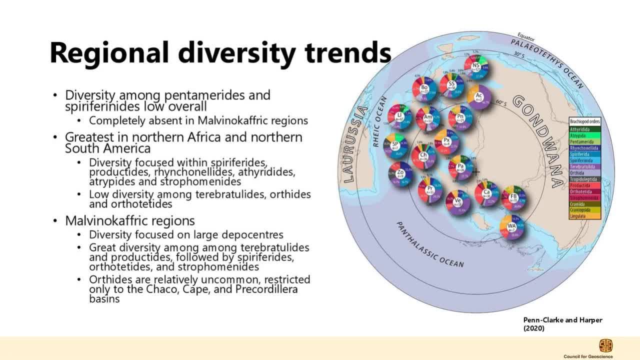 the greatest diversity is in northern Africa and north and south america, whereas in the southern regions, in the Malvino Capric realm, diversity was focused mainly on large depot centres. so the Cape, the Ventana and the Chako and the Paranna, but and also all thoughts, oddly, are quite uncommon and not as diverse. so we 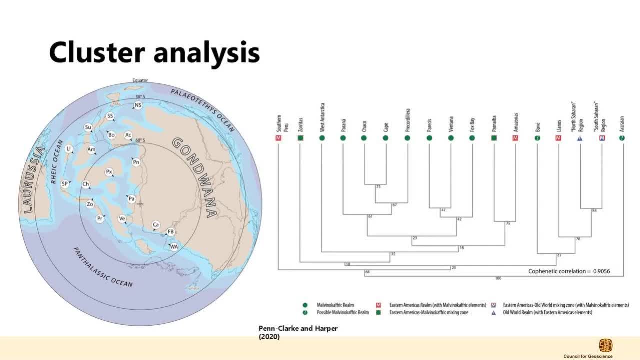 took a bunch of methods to actually try and reconstruct natural regions. we use cluster analysis and cluster analysis what showed quite nicely is that we could divide this into a high latitude region and a temperate latitude region, which you know fits the map quite nicely, and that it could be split down further. 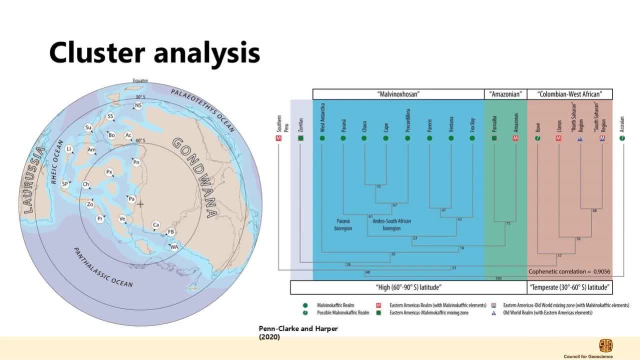 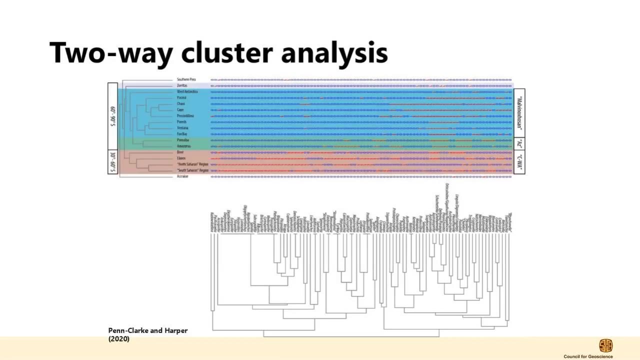 in the high latitude regions, the Malvina Malvina cause in fire region, Amazonian and the Colombian West African, and that one could see subdivisions within the Malvina cause in the piranha and up and do South African fire region and in the 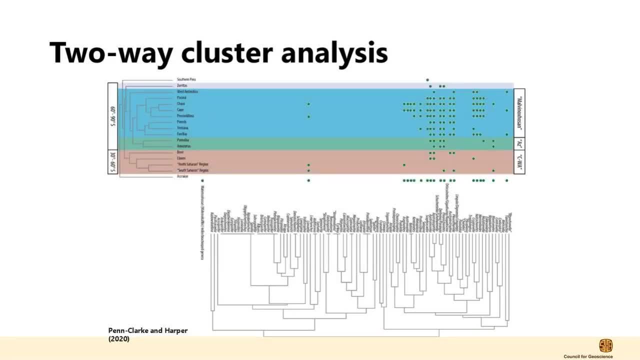 two-way cluster analysis: again we see the same thing as well. all these Malvina Catholic taxa tend to group together in more of these high latitude regions in Southwest and Gondwana and we looked also at non-metric multidimensional scaling to have a look. 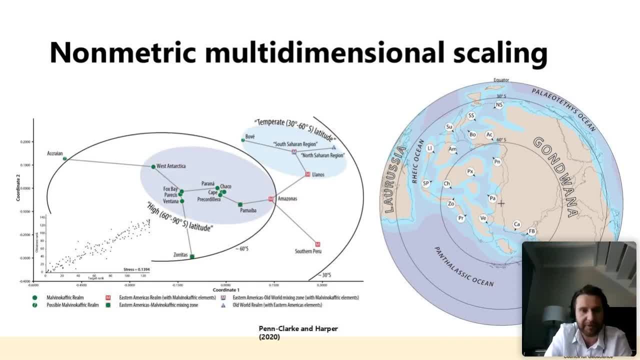 at the distances among these regions. and again, what we noticed is that you see this again, the same grouping according to latitude is that these higher, highest latitude regions tend to group together and the more temperate latitude regions group together as well. so I mean, this was just some more artistic sort of 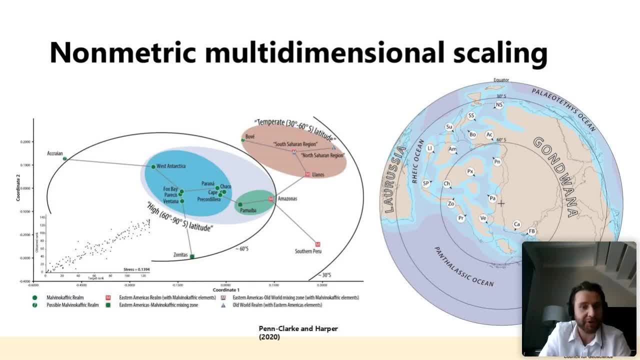 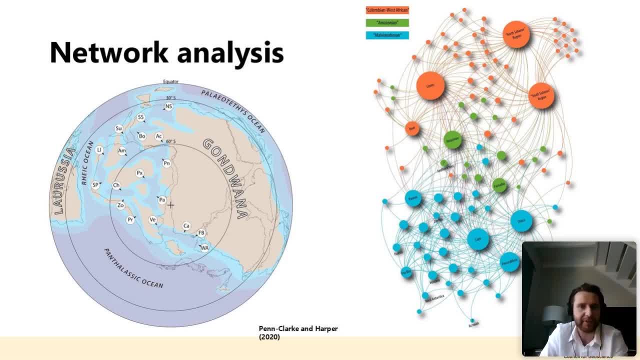 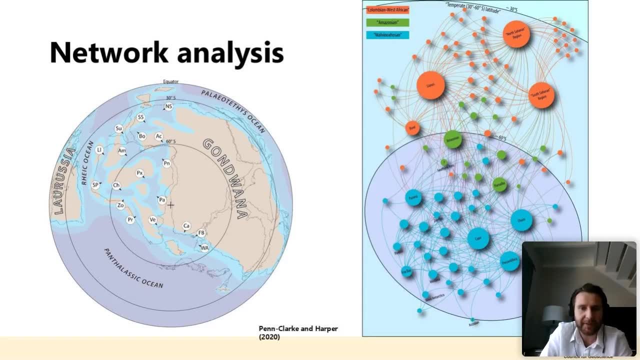 network analysis to make these very pretty pictures to let you look at the connectivity among these regions. and again, what we noticed as well is again that these regions also group, again according to inferred paleo-latitude. so again you could see a high latitude grouping, a temperate latitude grouping. 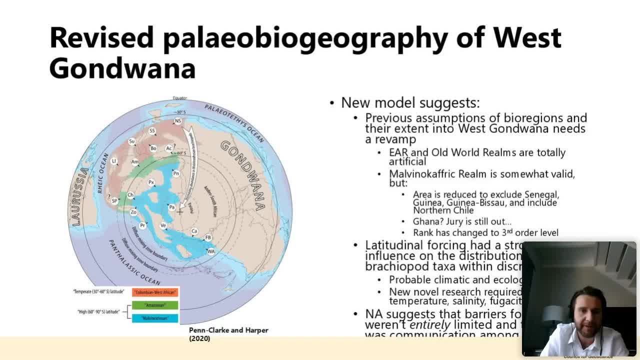 and groupings within the high latitude grouping. So the new model that we have suggests that previous assumptions for bioregions in West Gondwanan needs a revamp. So the East American realm and the Old World realms seem to be artificial. The Malvino-Catholic realm, however, 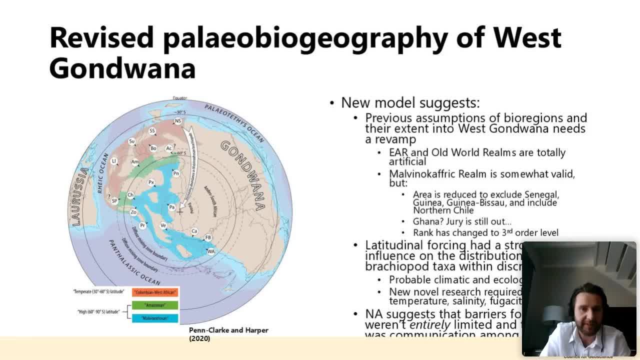 is valid, but with some adjustments, in that we could not reconcile whether Senegal, Guinea and Guinea-Bissau were part of the Malvino-Catholic realm, But Northern Chile seems to make the cut. Ghana: we're not really sure where Ghana fits in that collecting is quite poor from that region. 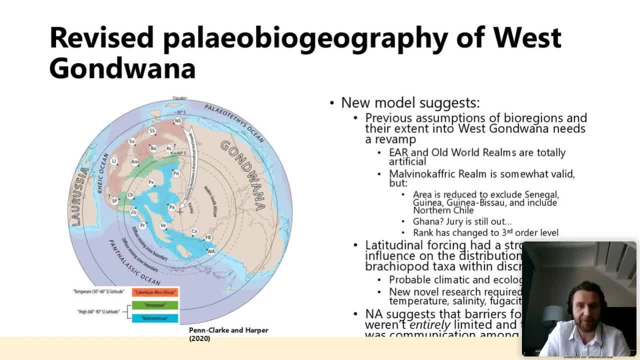 So we're hoping to go there in the future, when things hopefully get better, to go and actually have a look at this again. So latitudinal forcing seems to have had a strong influence on the district Latitudinal brachiopod taxa and that they occurred within discrete climatic vaults. So 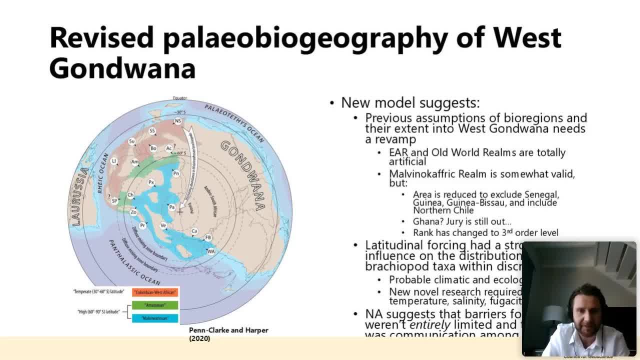 there were probably climatic and ecological effects that were associated with this, But that these barriers were. we can see from the network analysis that these barriers weren't true allopatric barriers, that they were more porous barriers that one or two little guys were able to get through and back and forth. So these regions were in. 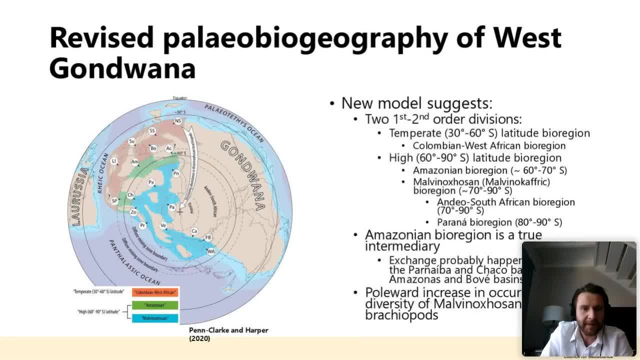 some form of communication with each other. So our new model that we are proposing: we have two large first-order divisions: a temperate latitude bioregion comprising entirely of the Colombian and West African bioregion, and a high latitude bioregion comprising the Amazonian bioregion and the Malvina Kauzan, which is a successor of the Malvina-Catholic bioregion, And at this bioregion- Canada and Malaysia- we have two large first-order divisions. The Central Asian and Western African bioregions are mostly different types of bioregions and we have high latitude bioregions and large 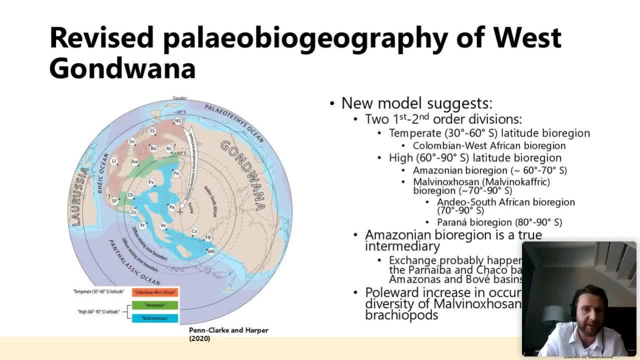 can be subdivided further into the andeo-south african bioregion and the piranha bioregion, which is located at the very highest latitude. so the amazonian is an intermediary and we see a forward increase in the occurrence and diversity of malvina cause and brachial parts towards the 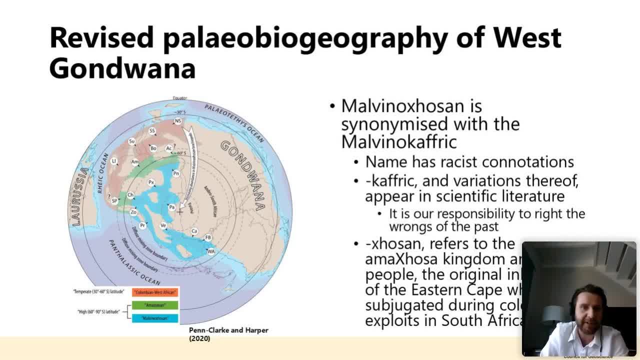 piranha. so why we have decided to change the name of the malvina catholic is that it has very racist connotations, um, and we are proposing that the catholic part changes to cause them to refer to the amakosa kingdom and her people, the original inhabitants of that region, um. 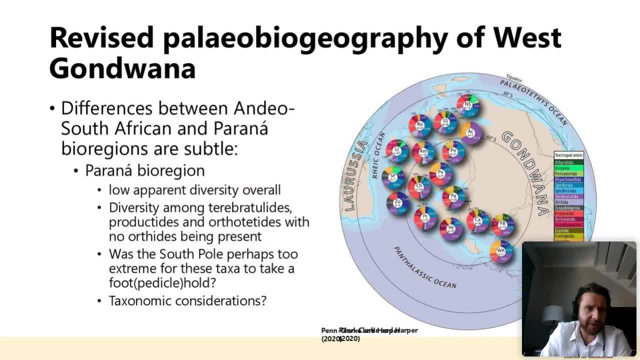 so further research that we are looking in the future now is to try and figure out, with the piranha region, the highest latitude subgroup of the, of the of the um, of in a cosmic bioregion. uh, why does it have a lower parent diversity overall um? were? was it perhaps too extreme for? 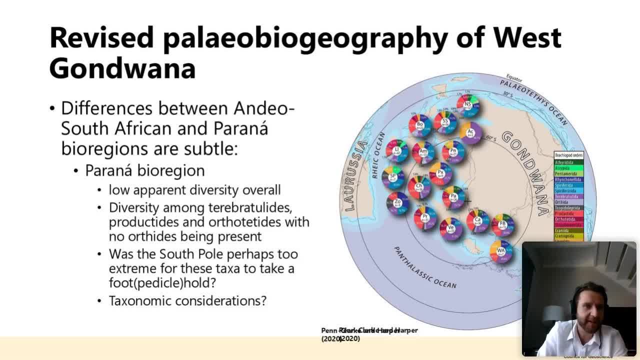 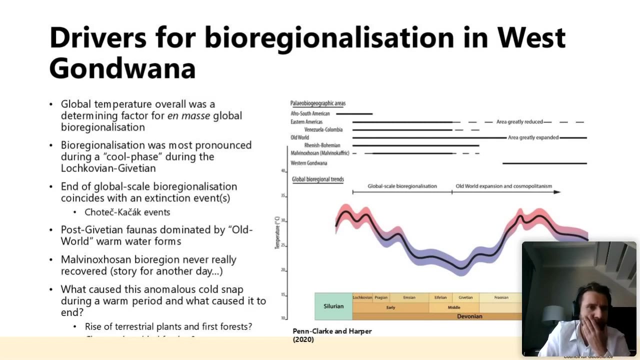 these taxes to take a pedicle hold on substrates, haha, um and um, yeah, because there's, uh, the the difference being is that, um, there are no author orthoids. product types and orthotetides are quite, um, not as quite diverse. um, and then, understanding the collapse of this, of these bioregions, is that global temperature. 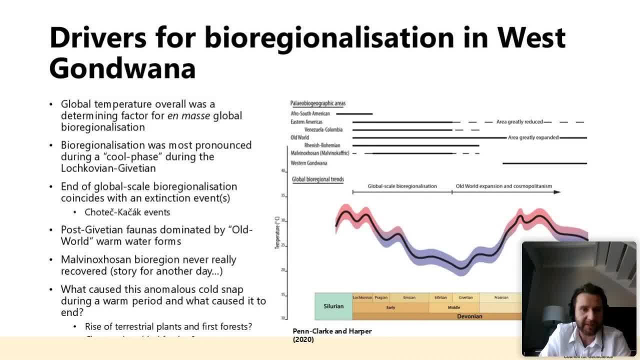 seems to have been a determining factor is that bioregionalism globally was during this cold phase, during the lakovian, south pelian, and with this warming from the gervetian onwards we see a collapse. so we are looking into this again. uh, later on this could be a large, this could be. 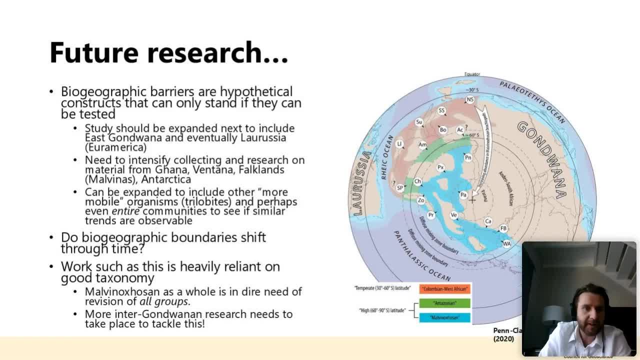 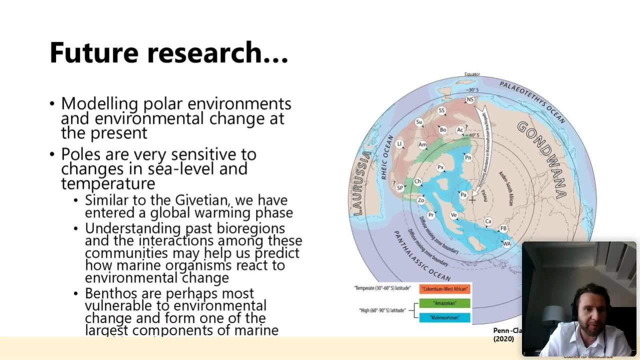 this is a more multi-faceted project, um, so, yes, we should look elsewhere in future. do these boundaries shift in through time? how do other regions fit into this where marvina cousin groups are found? um, and, yes, i'll just go through over here to do some more multi-proxy work, and this is important in that, yeah, these environments in the 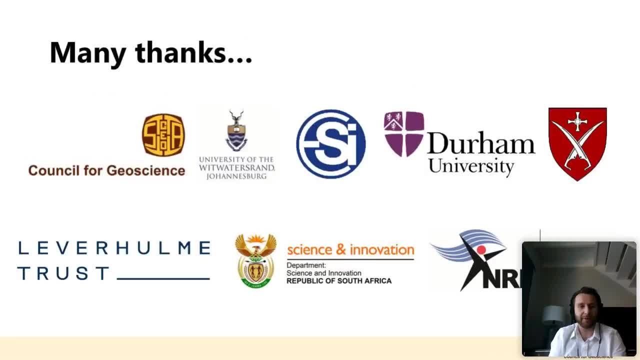 present day are quite fragile, so many thanks for your attendance today. i'd like to thank the council for geoscience, um, as well as durham university for for funding this project, making it possible when i was there as a visiting researcher, and our funders, leverholm trust, the dsi. 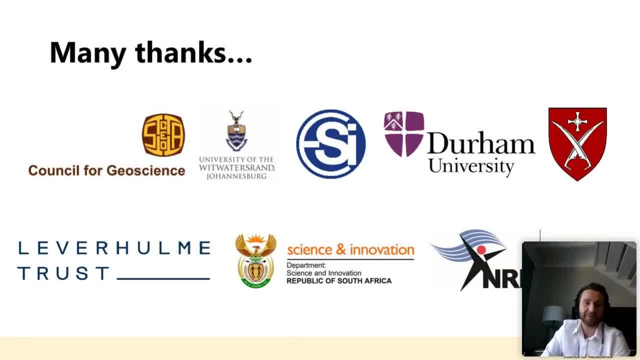 bits and the national research foundation. so thank you very much for making this possible. thank you so much, cameron, for that very interesting talk, and we have time for one quick question. please do keep writing some of your questions in the chat and cameron will answer them. 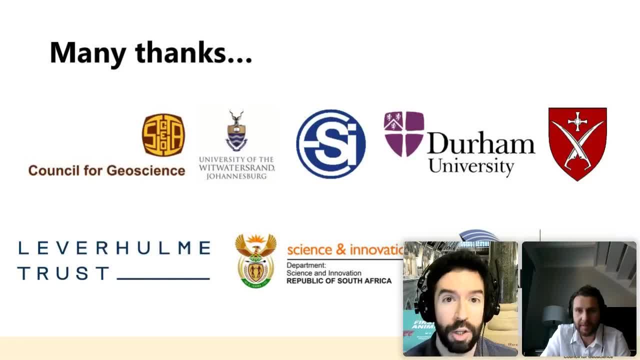 in the remaining of the session. so, based on your video biogeographical results, can you comment on the extent to which racquet larval stages stages are spread across the oceans within their given temperature tolerances of the adults that day? i have no answer for, to be honest with you, um, we are not at the point now.